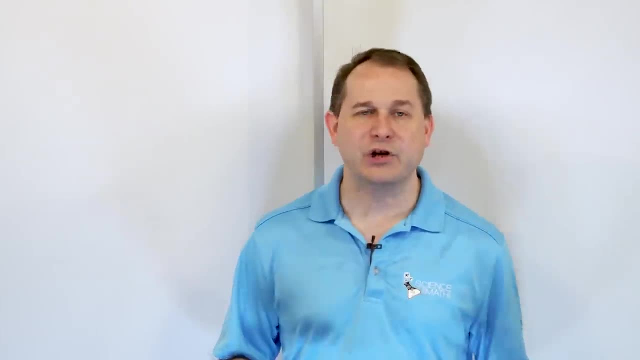 The exponent defines what the object is, just like the letter, And in math you can only add things if they're identical, like adding pencils to pencils. You can't really add pencils to dump trucks. I mean you can, but it doesn't going to make a lot of sense. So in math they have to. 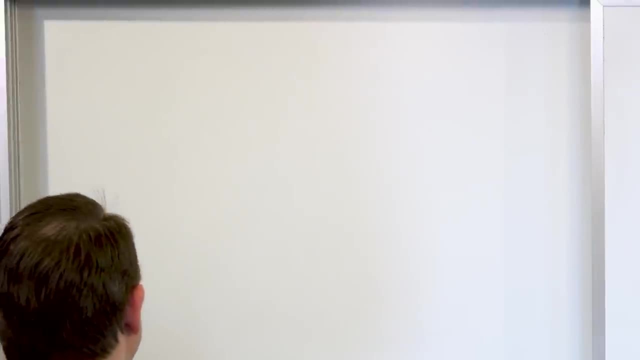 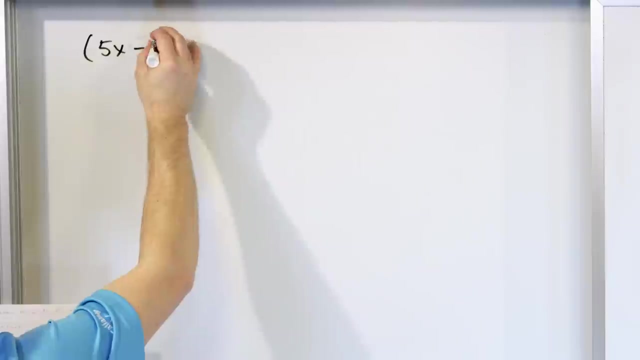 match exactly. So in order to jump into there and see how to do it, it's just much easier to do with examples. What if I had a polynomial 5x minus 4? That's a polynomial, In fact. what kind of. 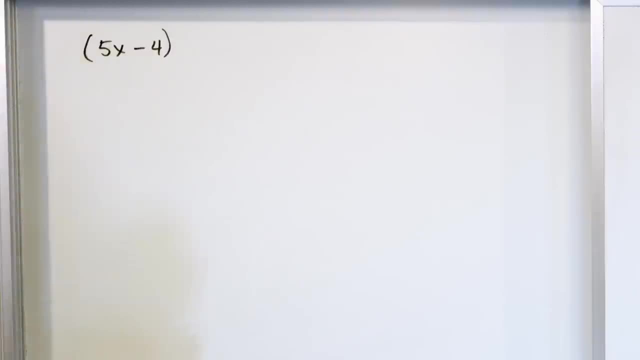 polynomial is this: You should know now that there's two terms, so this is called a binomial Plus. the next one is 2x plus 3.. All right, so that's another binomial. So we're adding a binomial to a binomial. Now, I've wrapped them in parentheses, because sometimes you see that. 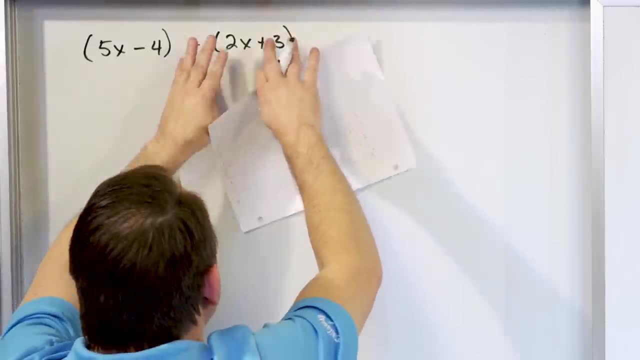 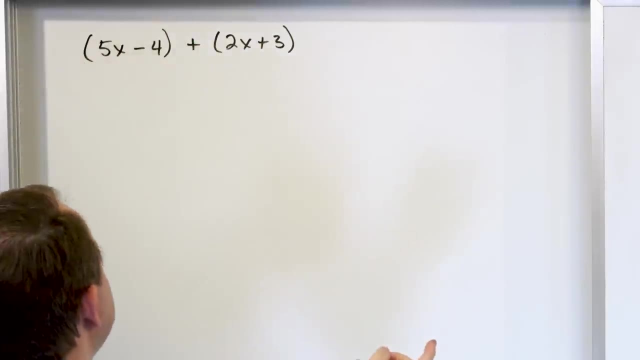 but also just to tell you that, hey, this is a polynomial and this is a polynomial and I'm adding them together. But in reality, since there's nothing outside of these guys to be distributed or multiplied in, then there's no real reason to have the parentheses there. if I'm 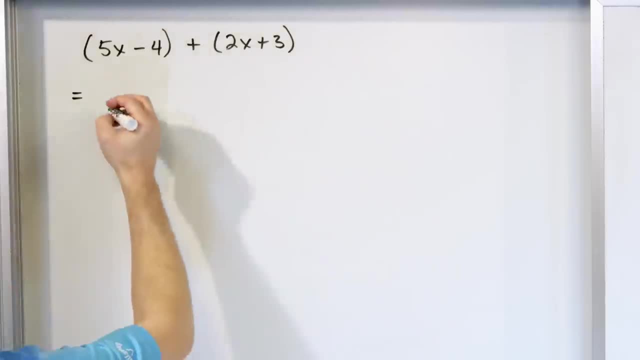 just going to add them. So, even though I wrote it in the problem statement, you can drop the parentheses and just write 5x minus 4 plus all of this stuff, 2x plus 3.. And, as I mentioned in the last lesson, what you're really looking for is like terms. This is an x to the power of 1. This 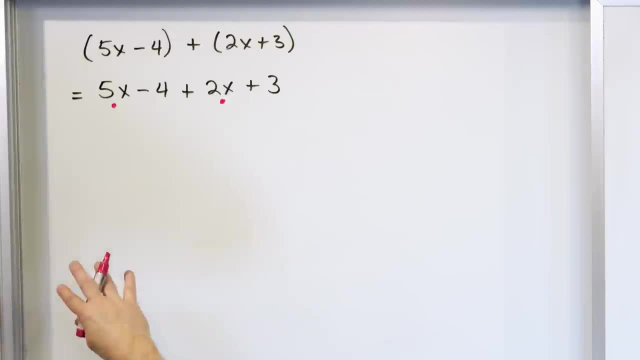 is an x to the power of 1.. And because of that I'm going to put a little dot under it to show myself that I've looked at these terms and I know that I can add them together. 5 plus 2 is 7.. 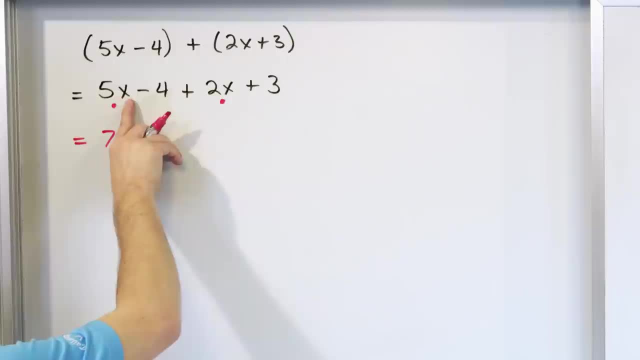 What am I adding? 7 x's, because here's 5 x's, Here's two more x's, And so when I put them together, I'm going to have x's. Now, that's the only variables that we have. So here we have a. 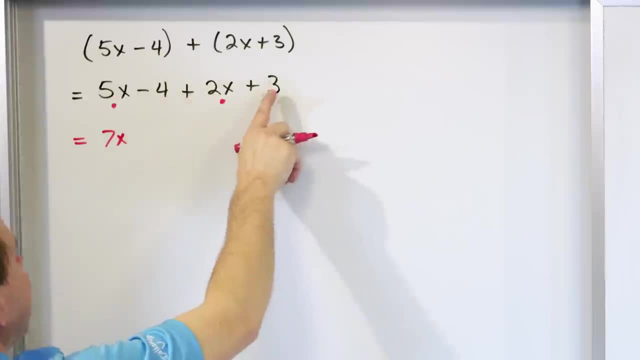 negative 4 and a positive 3.. You should know that negative 4 plus positive 3 is just negative 1.. Then the negative 1 goes at the end. So when you write the answer, you'll write the powers of x in decreasing format- In this case there's only one of them anyway- And then you have. 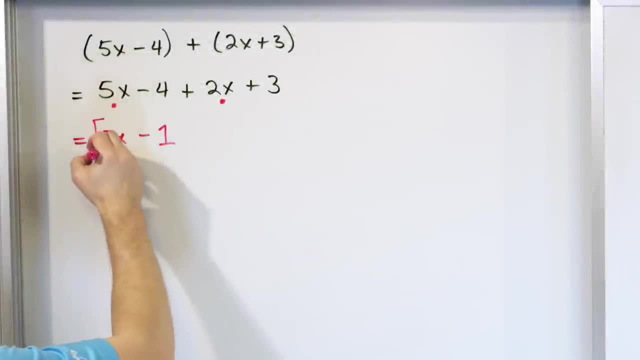 the minus 1 there And that's the final answer: 7x minus 1.. All right, So the next one. we're just going to mostly just crank through these guys. We're going to have increasing difficulty, go very slowly, increasing the complexity, But ultimately it's going to be the same thing every. 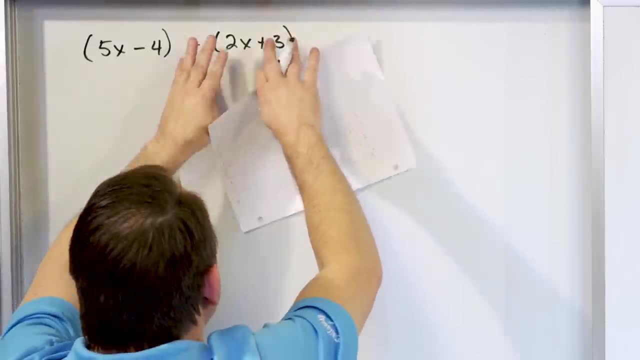 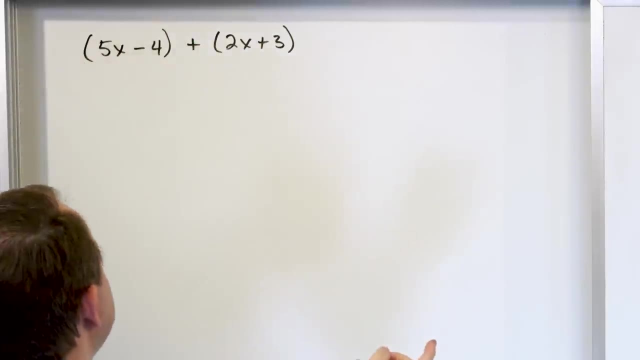 but also just to tell you that, hey, this is a polynomial and this is a polynomial and I'm adding them together. But in reality, since there's nothing outside of these guys to be distributed or multiplied in, then there's no real reason to have the parentheses there. if I'm 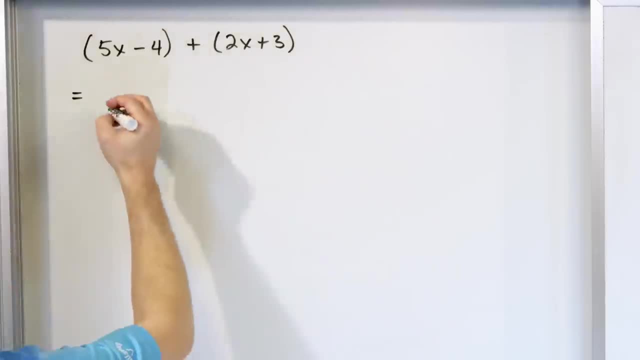 just going to add them. So, even though I wrote it in the problem statement, you can drop the parentheses and just write 5x minus 4 plus all of this stuff, 2x plus 3.. And, as I mentioned in the last lesson, what you're really looking for is like terms. This is an x to the power of 1. This 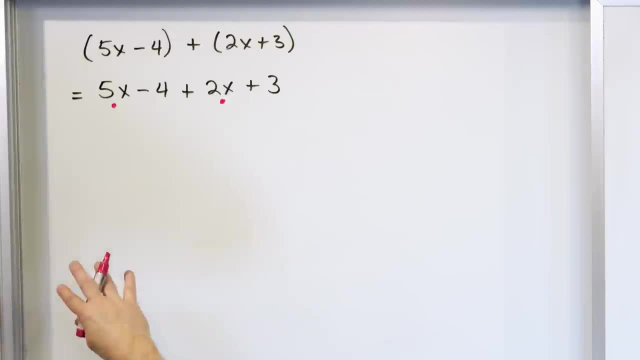 is an x to the power of 1.. And because of that I'm going to put a little dot under it to show myself that I've looked at these terms and I know that I can add them together. 5 plus 2 is 7.. 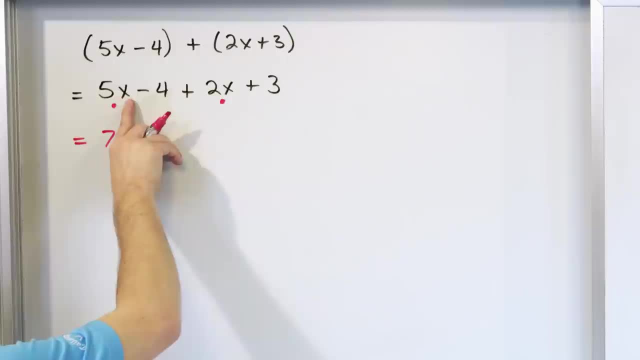 What am I adding? 7 x's, because here's 5 x's, Here's two more x's, And so when I put them together, I'm going to have x's. Now, that's the only variables that we have. So here we have a. 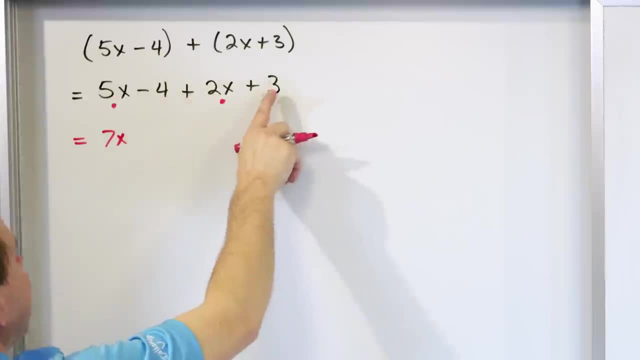 negative 4 and a positive 3.. You should know that negative 4 plus positive 3 is just negative 1.. Then the negative 1 goes at the end. So when you write the answer, you'll write the powers of x in decreasing format- In this case there's only one of them anyway- And then you have. 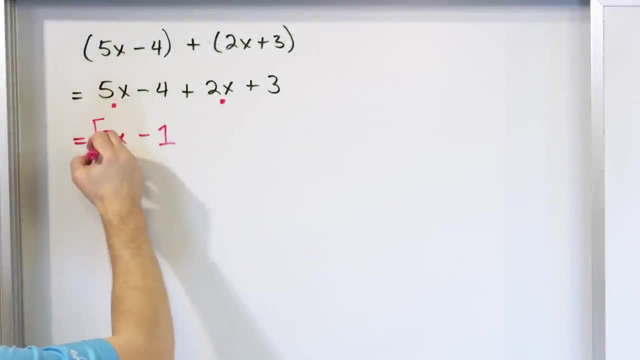 the minus 1 there And that's the final answer: 7x minus 1.. All right, so the next one. we're just going to mostly just crank through these guys. We're going to have increasing difficulty, very slowly increasing the complexity, but ultimately it's going to be the same thing. 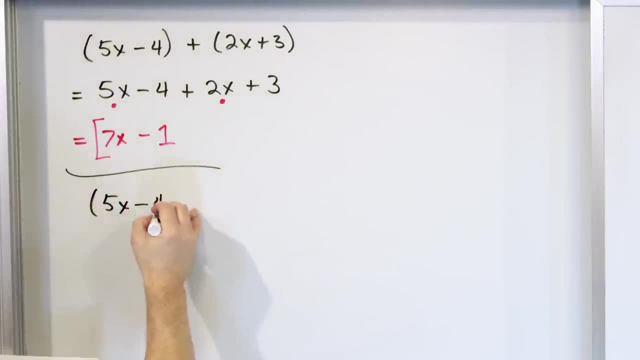 every time. What if we have 5x minus 4?? Now, instead of adding these polynomials, I'm going to subtract 2x plus 3.. Now you see, the difference between this guy is that they're linked with. instead of addition, this is subtraction. So the only way I can proceed. 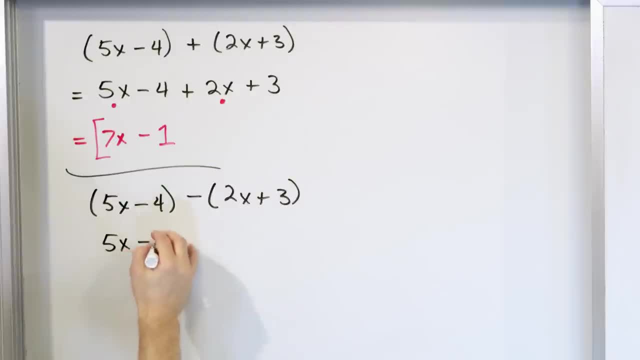 if I want to drop the parentheses. 5x minus 4, is this is a negative 1 on the outside. So this negative 1 needs to go in and multiply times this and then also times this. So I'm going to do this. So negative 1 times the 2x is going to give you negative 2x And the negative 1 times. 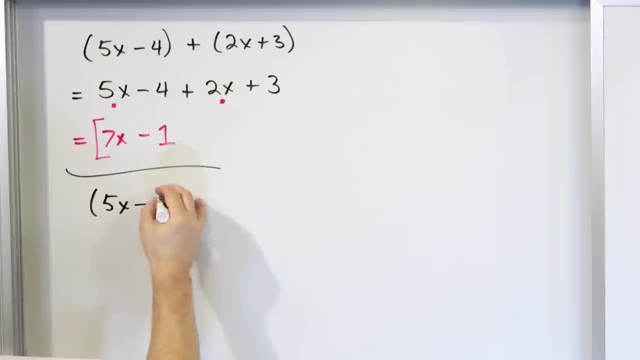 time. What if we have 5x minus 4?? Now, instead of adding these polynomials, I'm going to subtract 2x plus 3.. Now you see, the difference between this guy is that they're linked with instead of. 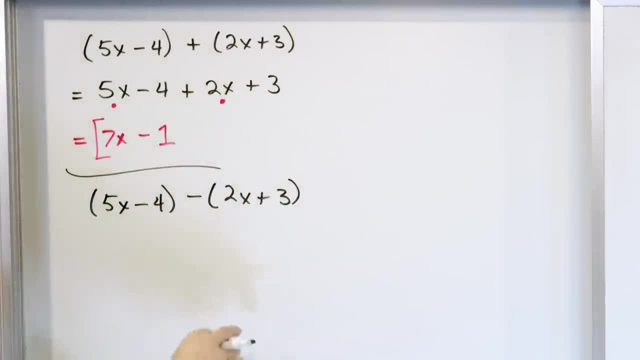 addition, This is subtraction. So the only way I can proceed if I want to drop the parentheses- 5x minus 4, is this is a negative 1 on the outside, So this negative 1 needs to go in and multiply times this and then also times this. So I'm going to subtract 2x plus 3. And I'm going to 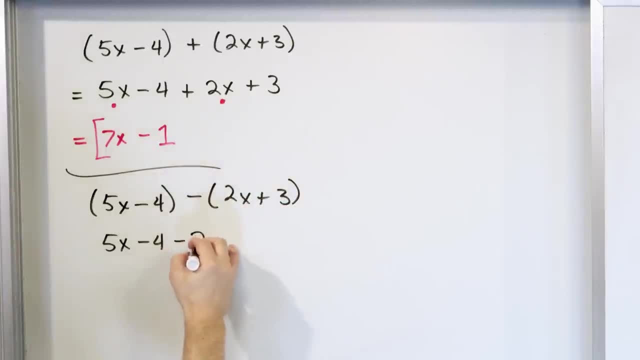 do this. So negative 1 times the 2x is going to give you negative 2x, And the negative 1 times the 3 is going to give you a negative 3.. Now I can add them If you just drop the parentheses. 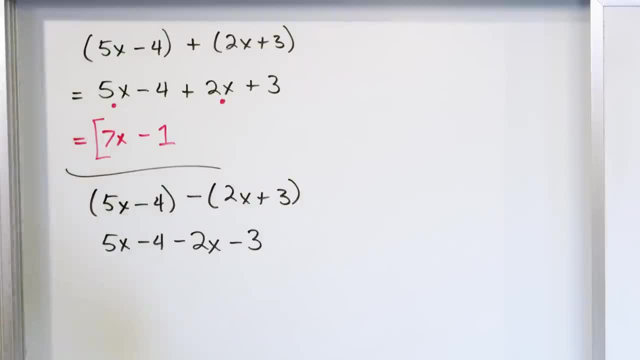 without distributing it, you won't have the proper signs everywhere and it won't work. So this is a negative 1. You have to distribute it in. Then I start looking for like terms. I have an x term here and I have an x term here. It's 5 minus- don't forget the minus sign- minus 2,. 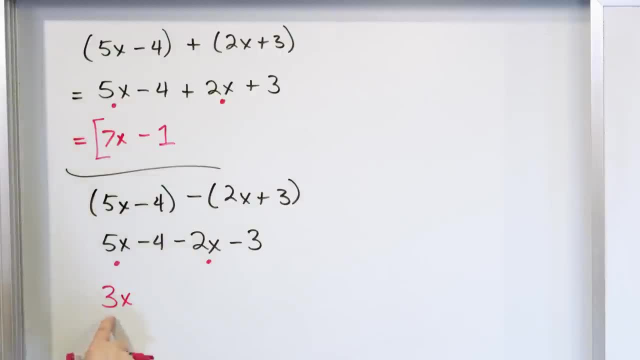 which is 3.. 3, what 3x terms? So that deals with the first part. And then I'm going to, just for clarity, I'm going to write the minus 4 here and I'm the minus 3 here. 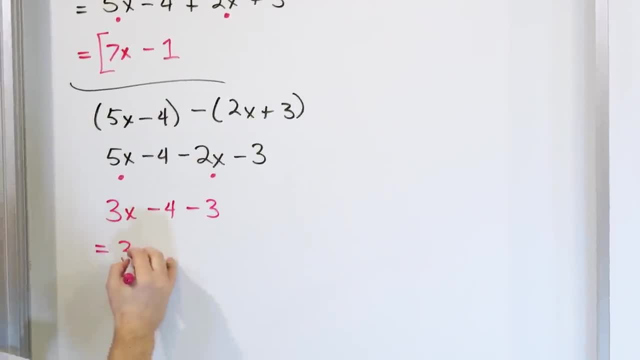 I'm not going to do that until the next step. Just to make it absolutely clear: I have 3x. What's negative 4? Minus 3 is negative 7.. So it's 3x minus 7.. That's the final answer. 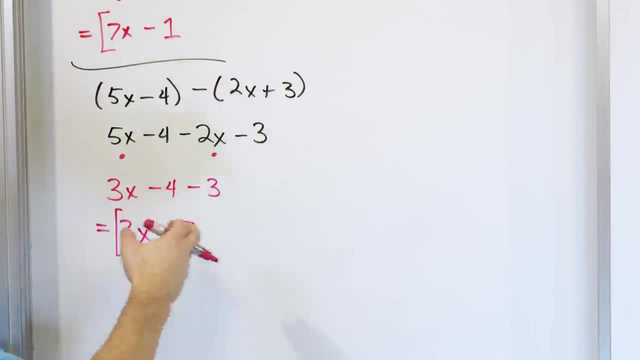 So you look for x terms that match and then you look for the numbers that match and pretty much we're going to be doing the same thing over and over again. No real difference. Let's take a look at the next one. It's going to look more complicated. 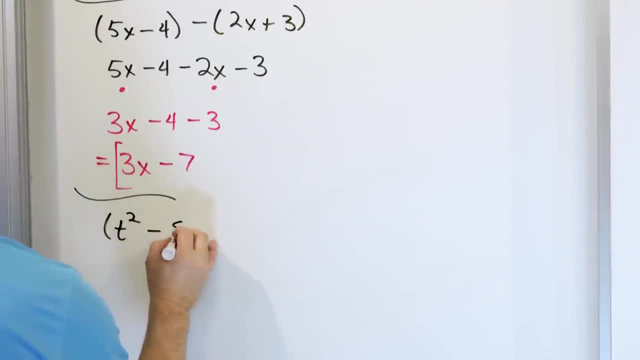 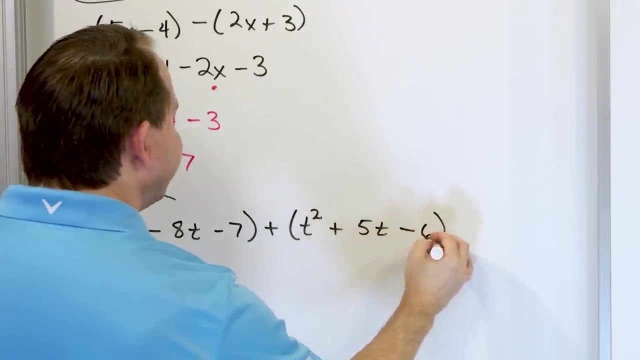 t to the power of 2.. t to the power of 2 minus 8 times t. Let's see here Minus 7, and then plus t squared, plus 5 times t, minus 6.. Now one thing I'm going to mention to you. I don't always do this, but I'm going to mention it to you. 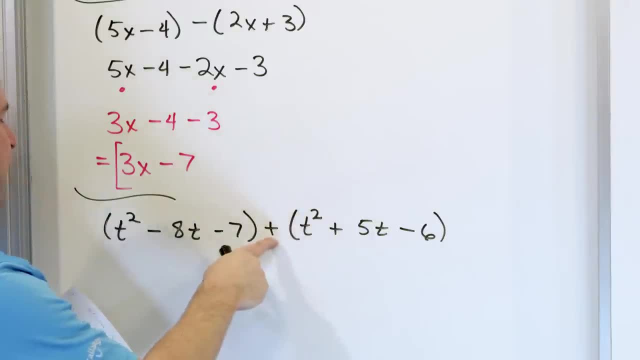 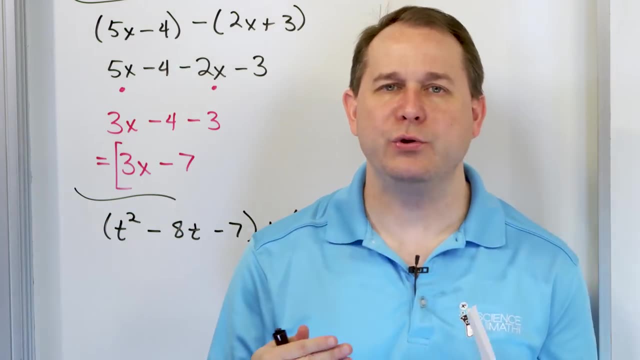 Notice that my plus sign is a straight up and down plus, But all of my t's have this little hook at the end: Hook, hook, hook, hook. I guess you can probably guess why. If you look at your t's as little plus signs, then you're eventually going to get confused when you have pluses everywhere. 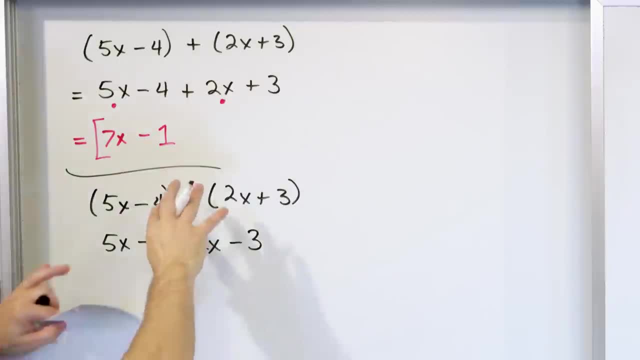 the 3 is going to give you a negative 3. Now I can add them. If you just drop the parentheses without distributing it, you won't have the proper signs everywhere and it won't work. So this is a negative 1. You have to distribute it in. Then I start looking for like terms. 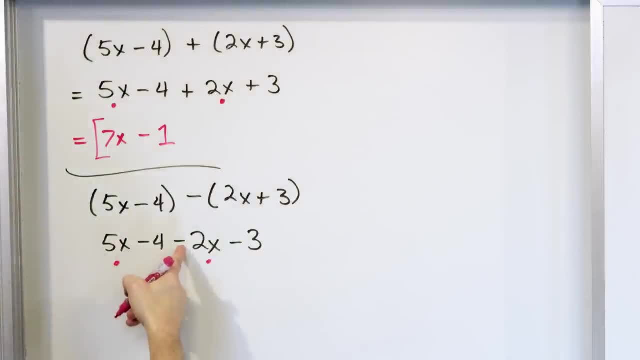 I have an x term here and I have an x term here. It's 5 minus- don't forget the minus sign- minus 2, which is 3.. 3, what 3x terms? So that deals with the first part. 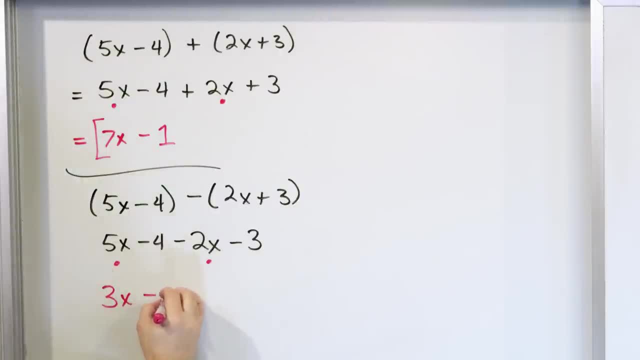 And then I'm going to. just for clarity, I'm going to write the minus 4 here and I'm the minus 3 here. I'm not going to do that until the next step. Just to make it absolutely clear, I have 3x. 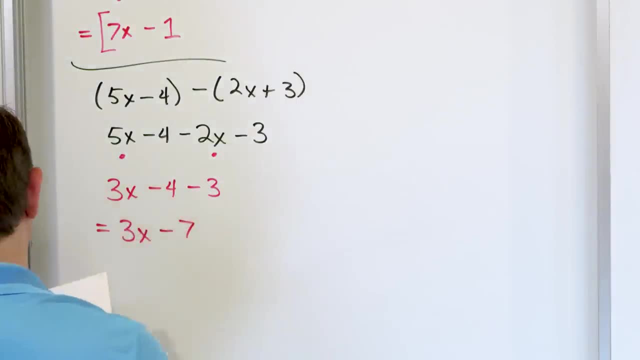 What's negative 4? Minus 3 is negative 7.. So it's 3x minus 7.. That's the final answer. So you look for x terms that match, and then you look for the numbers that match and pretty much we're going to be doing the same thing over and over again. 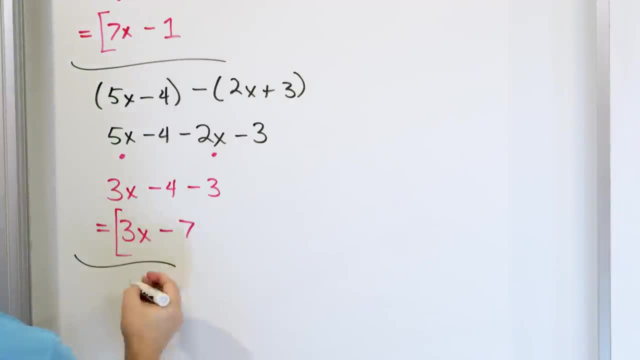 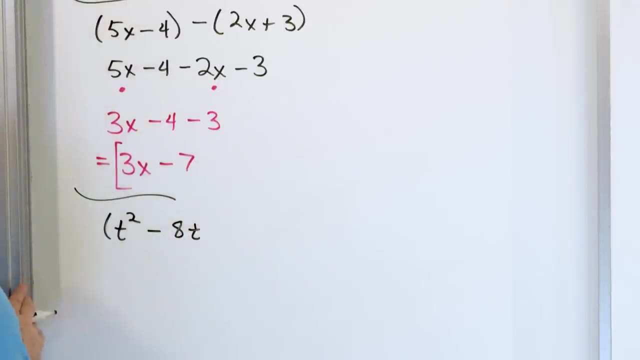 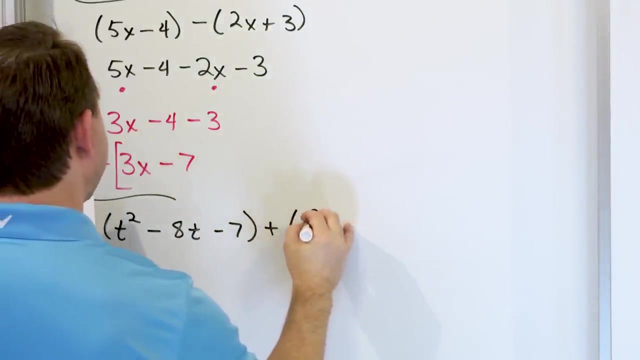 No real difference. Let's take a look at the next one. It's going to look more complicated. t to the power of 2.. Minus 8 times t, let's see here minus 7, and then plus t squared plus 5 times t minus 6.. 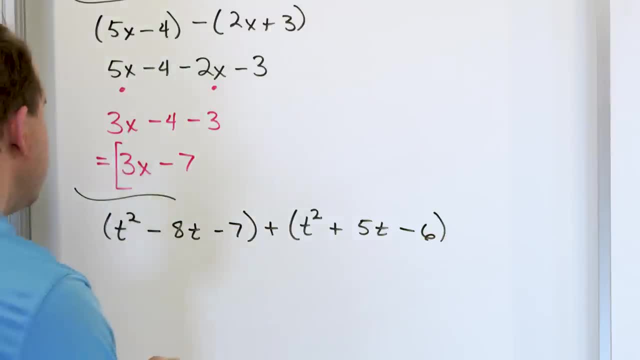 Now one thing I'm going to mention to you. I don't always do this, but I'm going to mention it to you. Notice that my plus sign is a straight up and down plus, but all of my t's have this little hook at the end: Hook, hook, hook, hook. I guess you can probably guess why If you just write your. 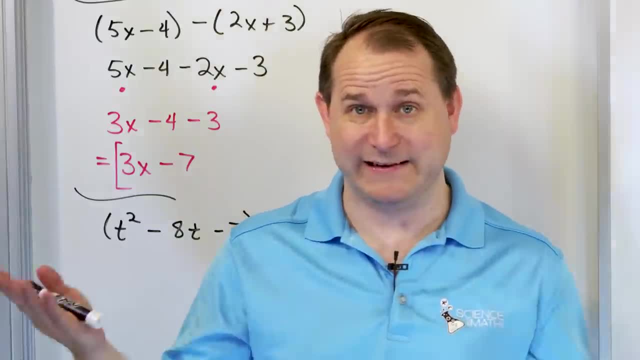 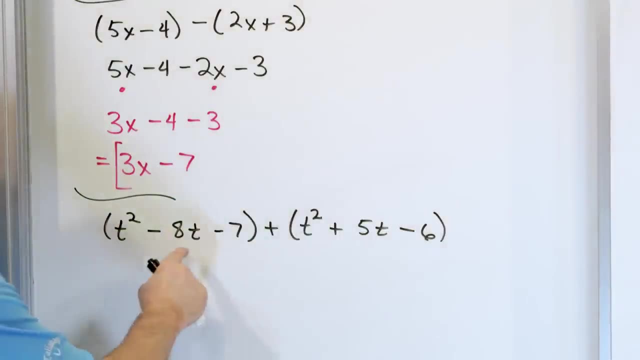 t's as little plus signs, then you're eventually going to get confused. When you have pluses everywhere, you're not going to know if it's the variable t or if it's a plus sign. So a long time ago I got in the habit of hooking my t's at the bottom. So if I'm dealing with a 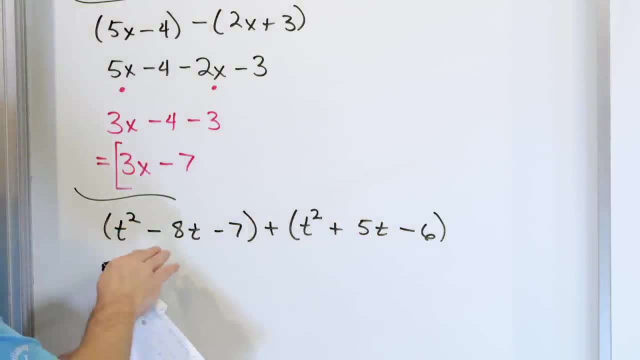 variable t. I always write it like that And I would encourage you to do that, because eventually you'll have a large equation with plus signs and t's and you can see how confusing it would be if you didn't make a distinction there. Now, this is a plus sign, so yeah, you're distributing the. 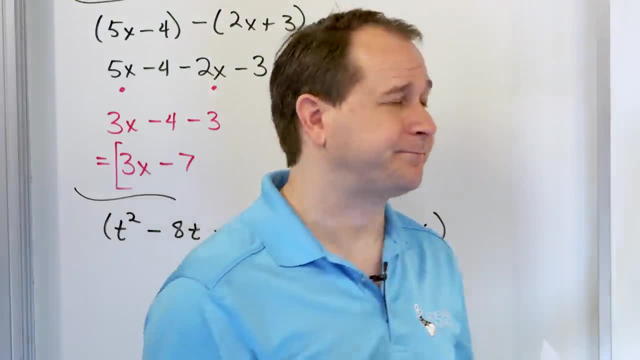 You're not going to know if it's the variable t or if it's a plus sign. So a long time ago I got in the habit of hooking my t's at the bottom. So if I'm dealing with a variable t, I always write it like that. 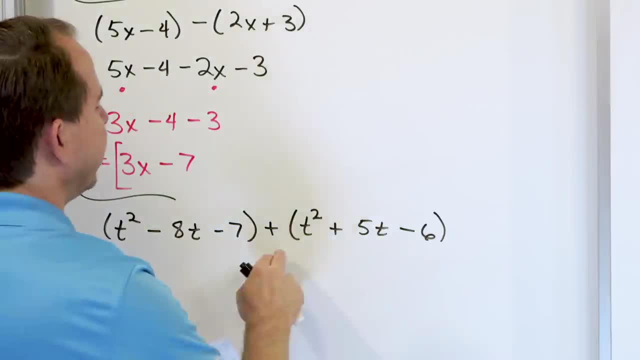 And I would encourage you to do that, because eventually you'll have a large equation with plus signs and t's and you can see how confusing it would be if you didn't make a distinction there. Now, this is a plus sign, So yeah, you're distributing the positive one in, but it doesn't make any difference. 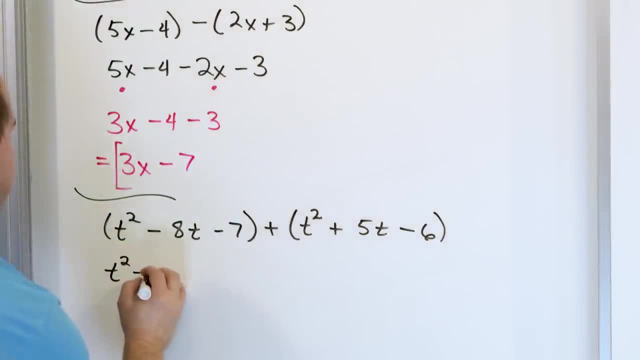 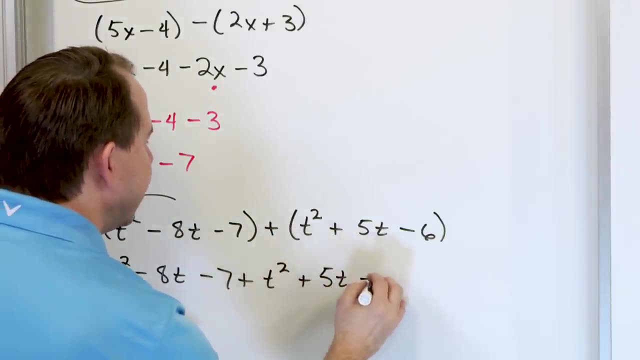 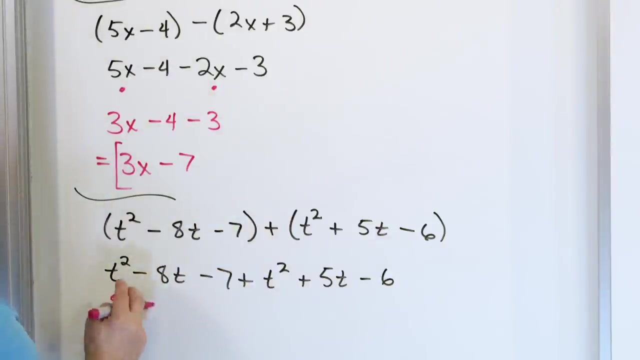 So what I'll do next is I'll just drop the parentheses: t squared minus eight, t minus seven plus here. t squared plus five, t minus six, And then I look for like terms. The largest power of t I have is the t squared here. 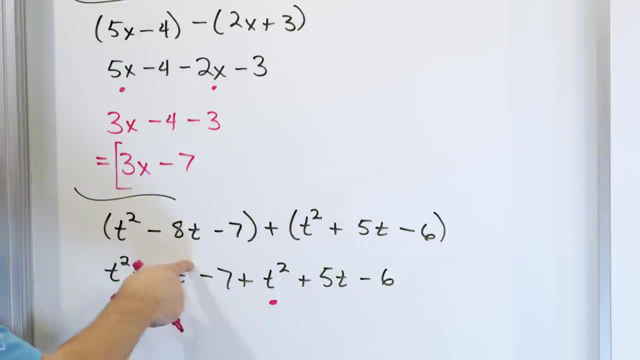 And I look for other like terms. Here's another one. This is not a like term because it doesn't have a square. This is not a like term because it doesn't have a square, So I can add these: One plus one gives me two, Two, what Two? t squares. 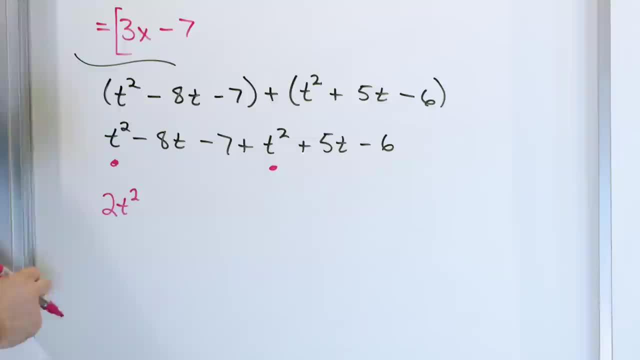 Here's a t square. Here's a t square. You add them together And I get two of them. Then the next thing I'll do- I'll switch colors to make this a little clear- is I'm going to look for t terms. 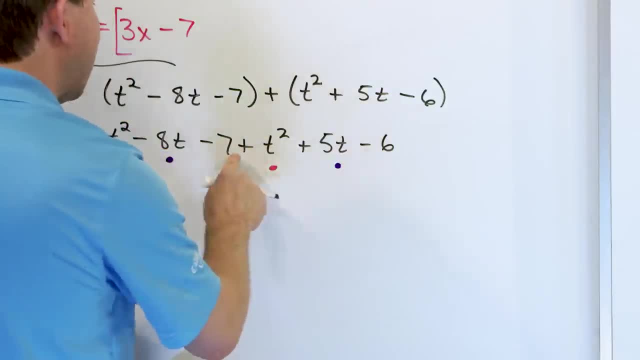 There is a t term And then I keep going, Here's another t term. Obviously, I can't add it to the numbers because there's no t's there, But here I have negative eight Right here. Let me think about this. Maybe the best way to do it is to rewrite things. I'll rewrite it again. 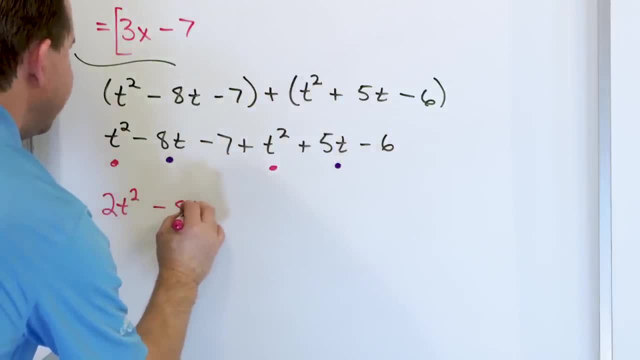 Let me go ahead and say this is going to be negative: eight t minus the seven plus the five t minus six. So all I've done here is I've added the t squares And then everything else is just coming down. I haven't done anything yet. 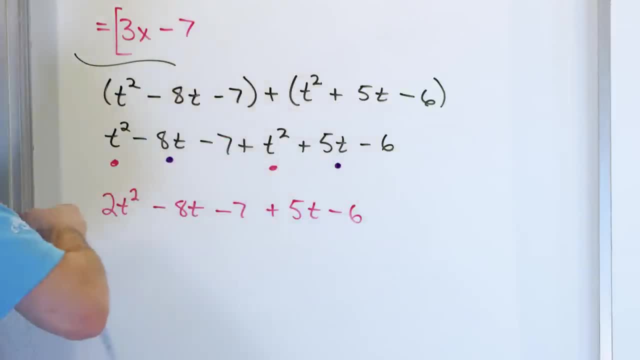 But now I look and say I have the negative eight and I have the five t. So what I'll do for that one is I'll say I have the two t squared. That doesn't change What is negative eight plus positive five. Negative eight plus positive five is negative three. Negative three times t. 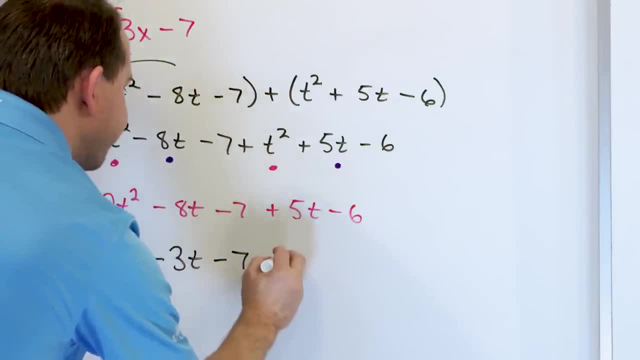 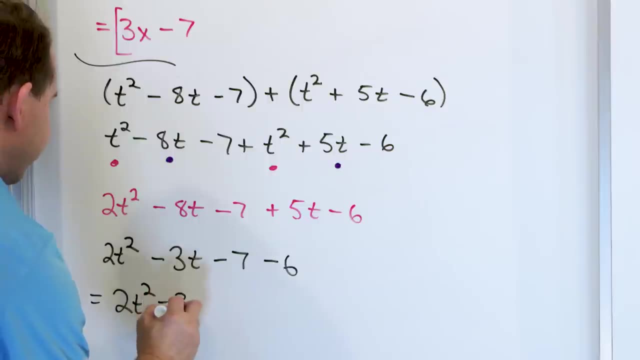 But I still have these numbers And let me just carry them on for now. Minus six. Negative seven here, Negative six. I'm not going to do this forever, But here in the beginning I think I can do that. Two t squared minus three times t, What is negative? seven minus six. 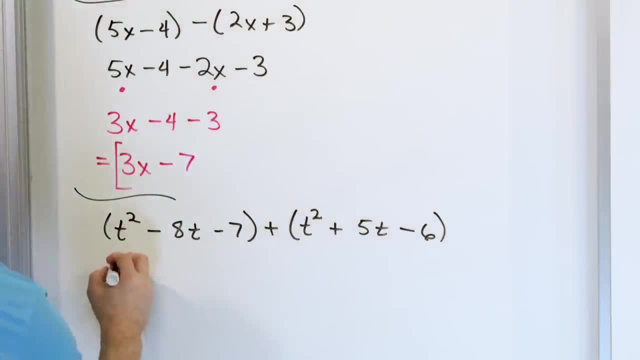 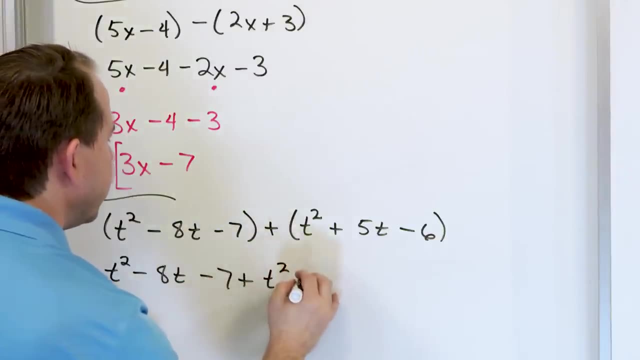 positive one in, but it doesn't make any difference. So what I'll do next is I'll just drop the parentheses. t squared minus eight, t minus seven, plus here: t squared plus five, t minus six. And then I look: 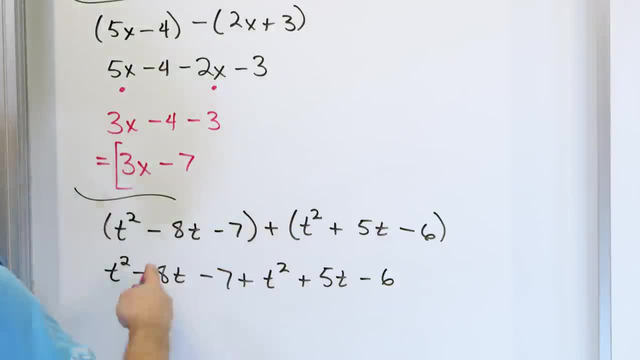 for like terms. The largest power of t I have is the t squared here And I look for other like terms. Here's another one. This is not a like term because it doesn't have a square. This is not a like term because it doesn't have a square, So I can add these. One plus one gives me two. 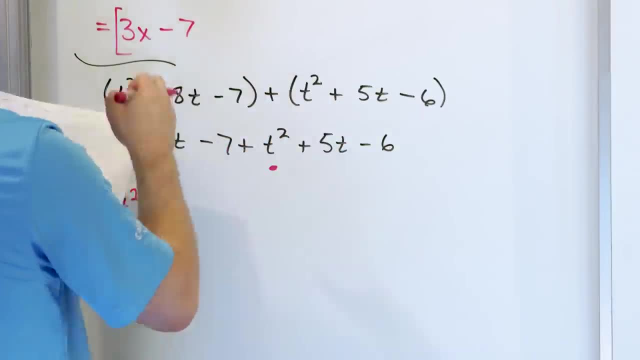 Two, what Two t squares. Here's a t square, Here's a t square. You add them together and I get two of them. Then the next thing I'll do- I'll switch colors to make this a little clear- is I'm going to look for t terms. There is a t term And then I keep going. Here's another t. 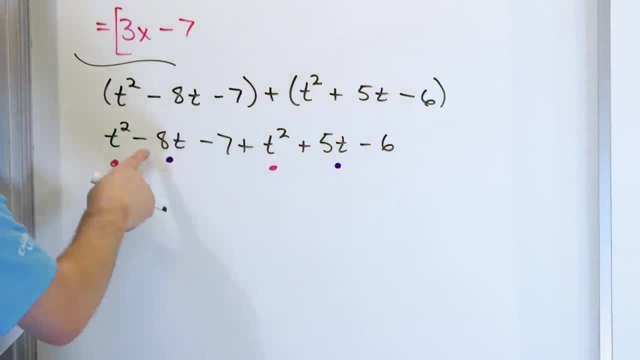 term. Obviously I can't add it to the numbers because there's no t's there. But here I have negative eight right here. Let me think about this. Maybe the best way to do it is to rewrite things. I'll rewrite it again. Let me go ahead and say this is going to be negative eight t minus. 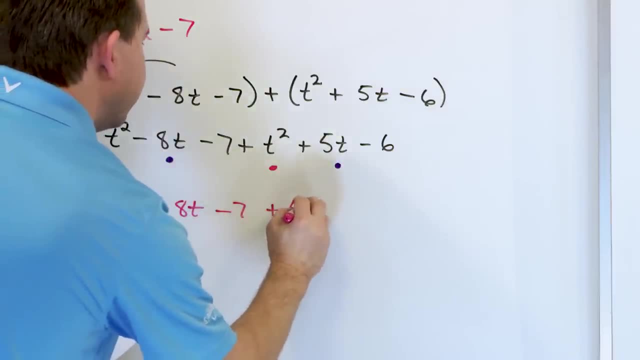 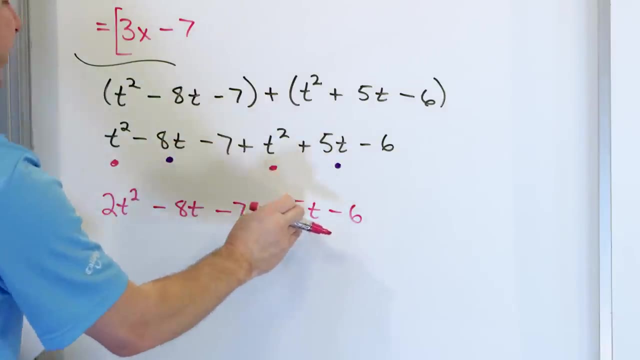 the seven Negative five t minus six. So all I've done here is I've added the t squares And then everything else is just coming down. I haven't done anything yet. But now I look and say I have the negative eight and I have the five t. So what I'll do for that one is I'll say I have the two t squared. 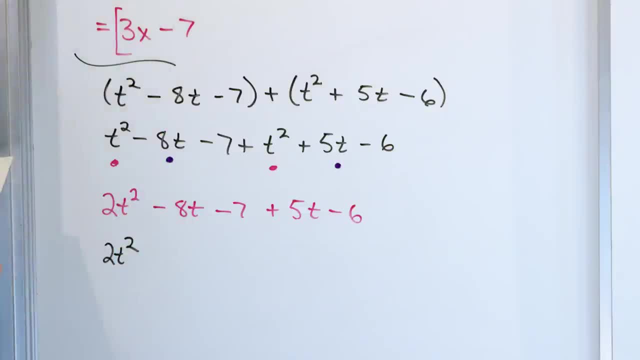 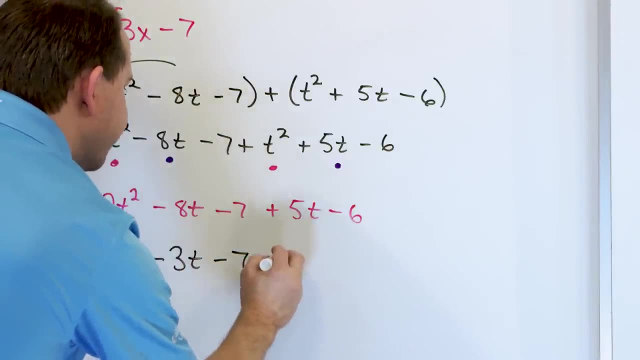 That doesn't change What is negative. eight plus positive five. Negative eight plus positive five is negative three Negative three times t. But I still have these numbers And let me just carry them on for now. Minus six Negative seven here. 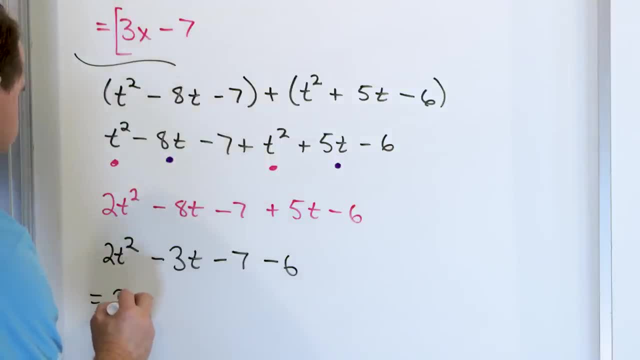 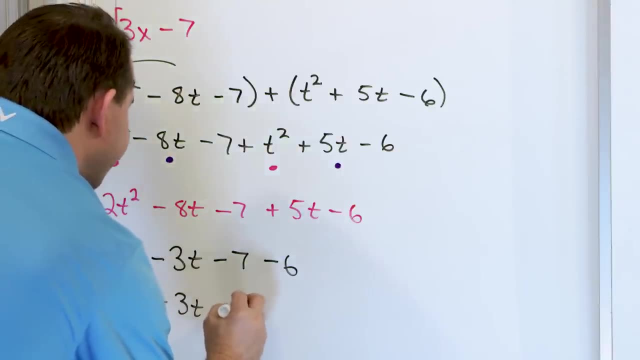 Negative six. I'm not going to do this forever, But here in the beginning I think I can do that. Two t squared minus three times t, What is negative? seven minus six, It's going to give you negative 13.. Because seven plus six is 13. And you have the negatives there. So you have two t squared. 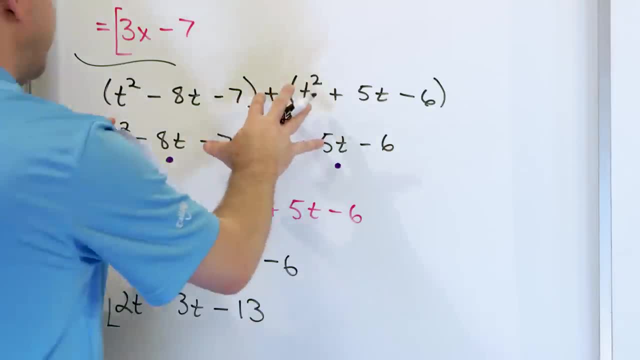 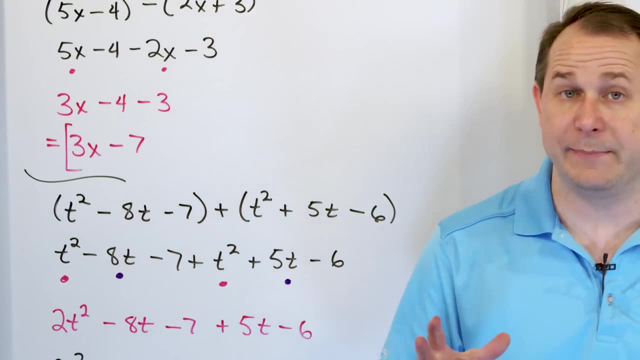 minus three t minus 13.. So again I showed every step, just adding each term along the way. I'm not going to do that forever because eventually it's going to slow you down too much. I mean I don't like skipping steps, But at the same time I need to kind of show you how you're really. 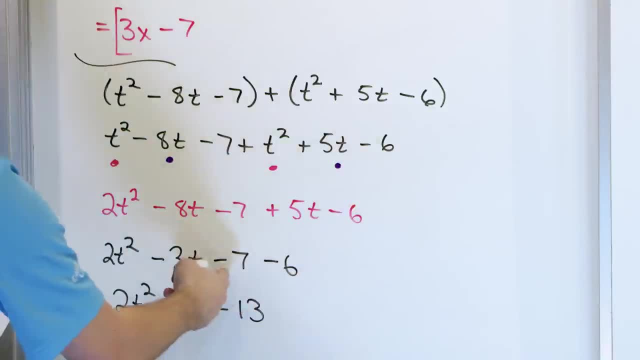 It's going to give you negative thirteen, Because seven plus six is thirteen And you have the negatives there. So you have two t squared minus three t minus thirteen. So again I showed every step, just adding each term along the way. I'm not going to do that forever because eventually it's going to slow you down too much. 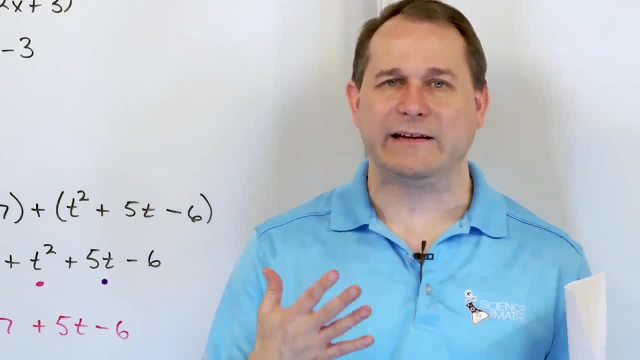 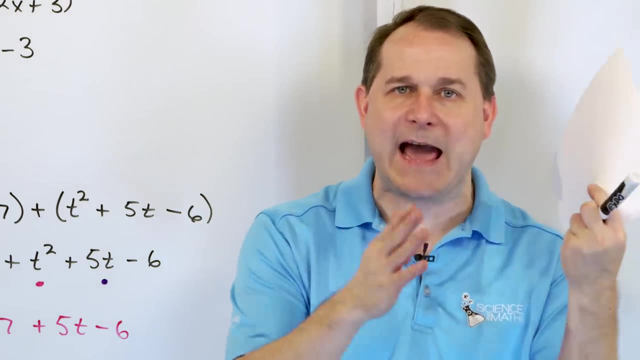 I mean, I don't like skipping steps, But at the same time I need to kind of show you How you're really going to do your homework. So in the first few problems I'll break it out like this, But after a few times we'll start kind of adding terms in parallel with one another. 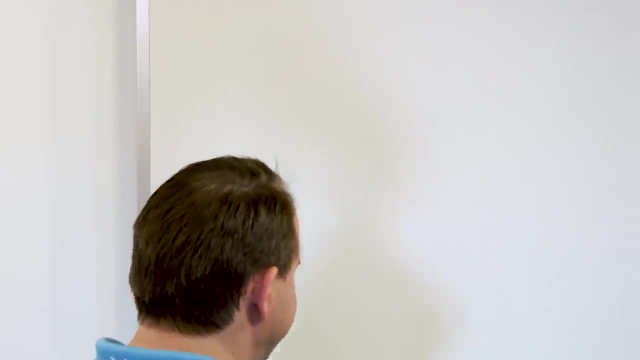 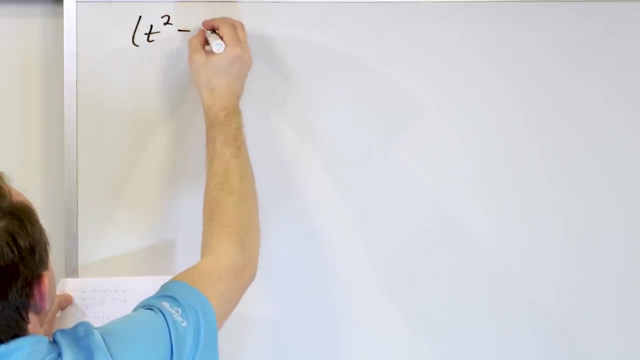 Just to show you how you really do it. So we're on to the next page. Let's take a look at the next set of polynomials to add together: What if we have t squared minus eight, t minus seven? We'll close that off as the first polynomial. 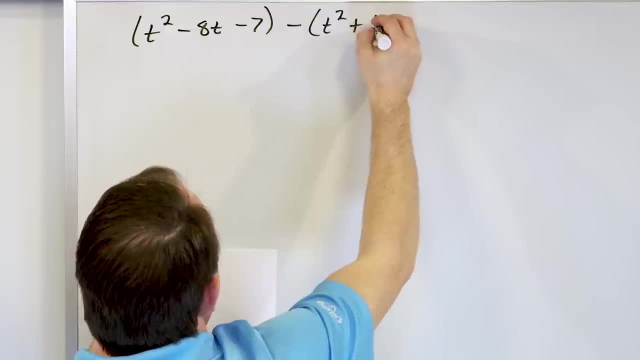 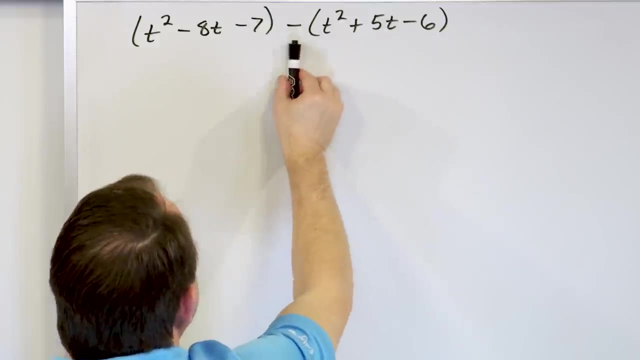 Minus t, squared plus five. t minus six, That's the second polynomial. Now notice critically that there's a minus sign. You're subtracting them, So the only way you can drop the parentheses is if you distribute the negative one in Multiplying times every term. 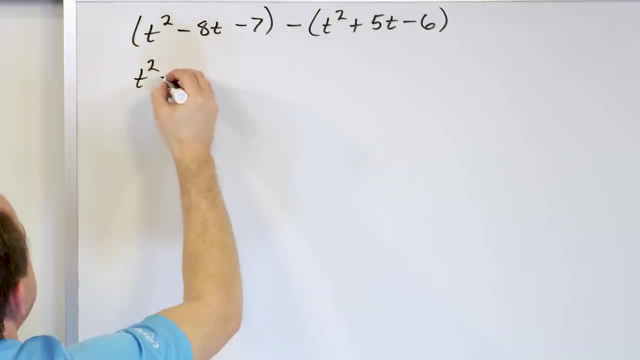 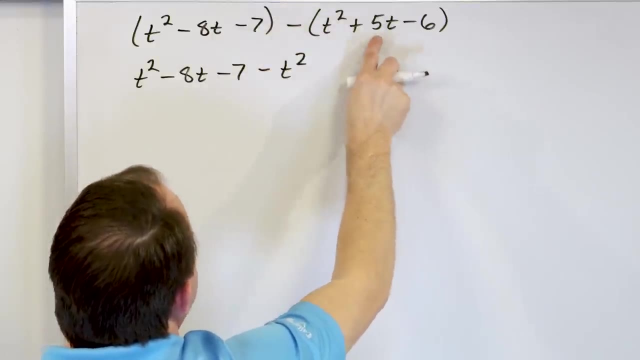 The first term is unaffected, So it's going to be t squared minus eight times t minus seven: Negative one times. this gives you negative t squared: Negative one times. this gives you negative five times t. Negative one times negative six gives you a positive six. 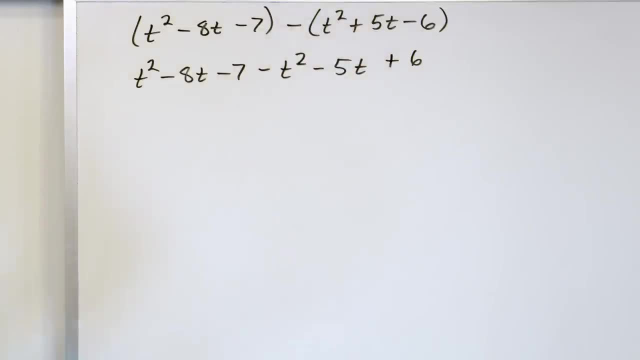 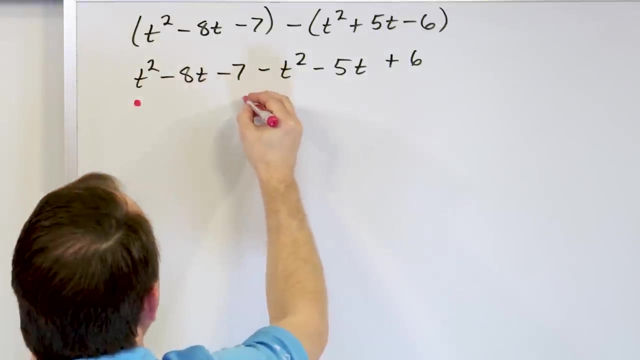 Don't forget that positive because of the multiplication here. And then I'm going to start looking at what I can add together. I have a t squared term here. I keep going. I have another t squared term here. I don't have any other t squareds. 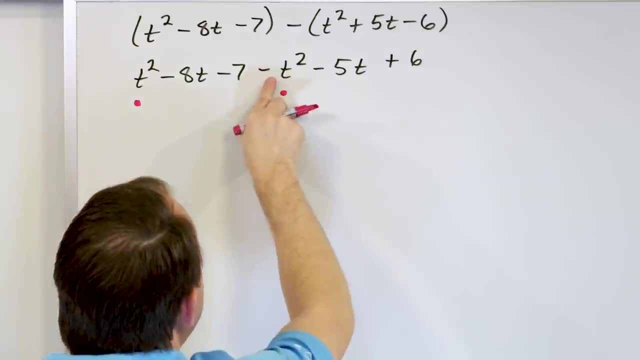 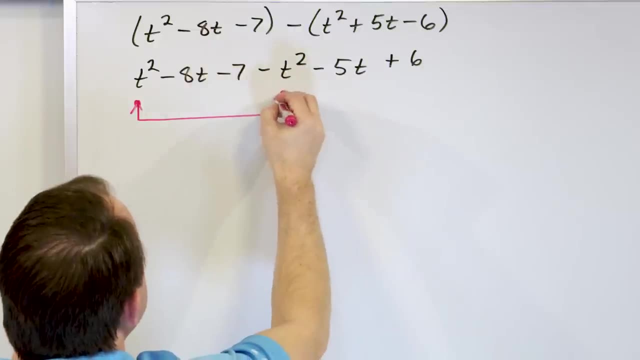 So I have a positive one minus one. So positive one plus a minus one, Or you can think of it as one minus one. So really, what's going to happen with these terms? it's going to give you zero. The t squares are going to disappear because it's one minus one. 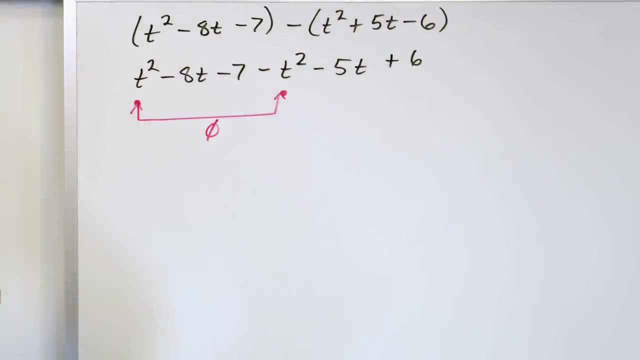 So they're going to disappear And just to have absolute clarity, I'm going to rewrite everything that's left over. This is left over. You're going to have negative eight t minus seven. The t squared's gone. Now we have minus five t plus six. 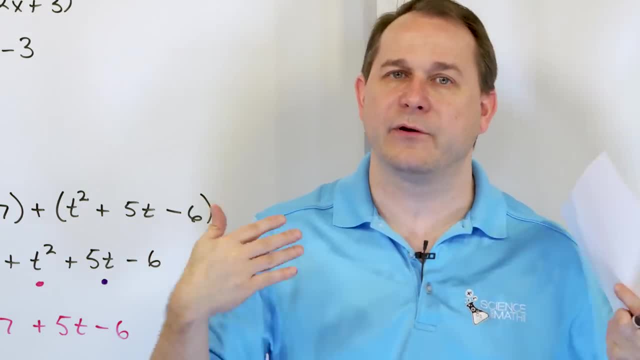 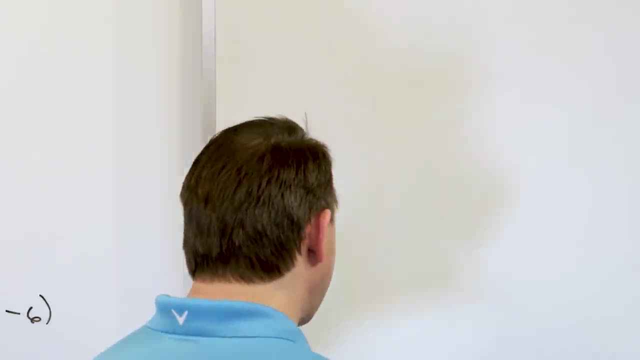 going to do your homework. So in the first few problems I'll break it out like this, But after a few times we'll start kind of adding terms in parallel with one another, just to show you how you'll really do it. So we're on to the next page. Let's take a look at the next set of polynomials. 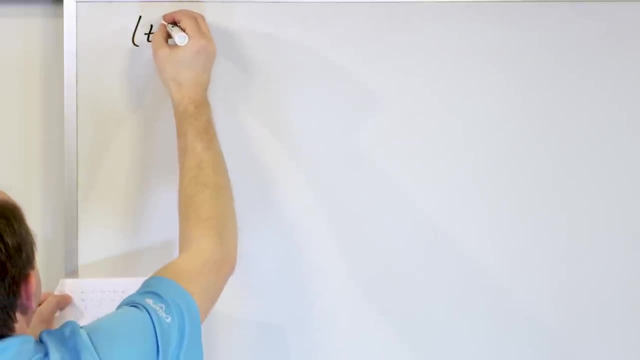 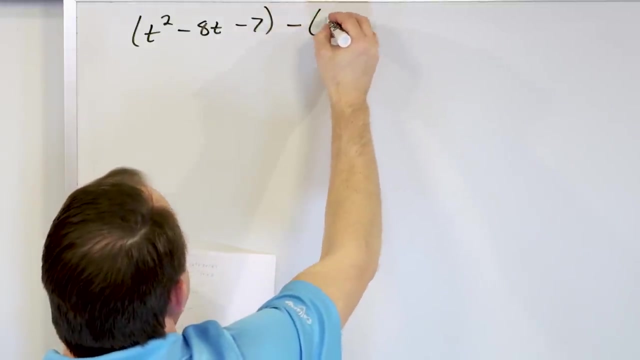 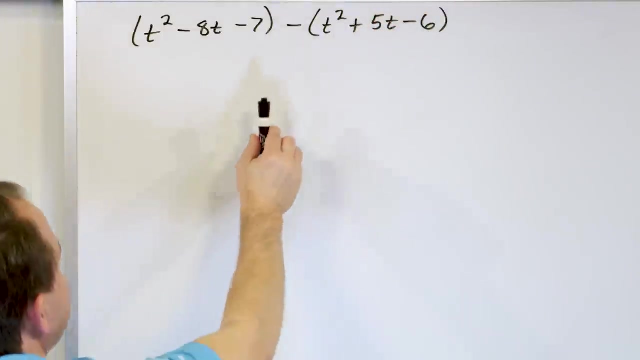 to add together. What if we have t squared minus eight, t minus seven? We'll close that off as the first polynomial Minus t squared plus five. t minus six. That's the second polynomial. Now notice critically that there's a minus sign. You're subtracting them, So the only way you can. 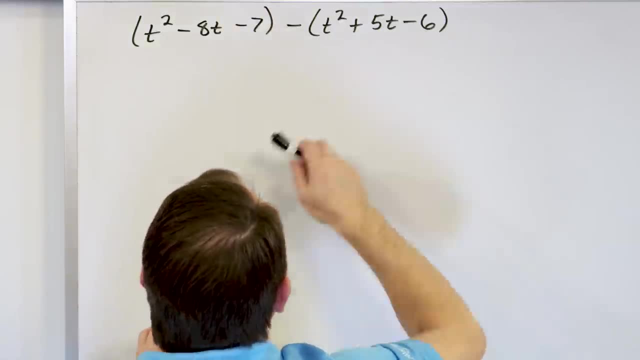 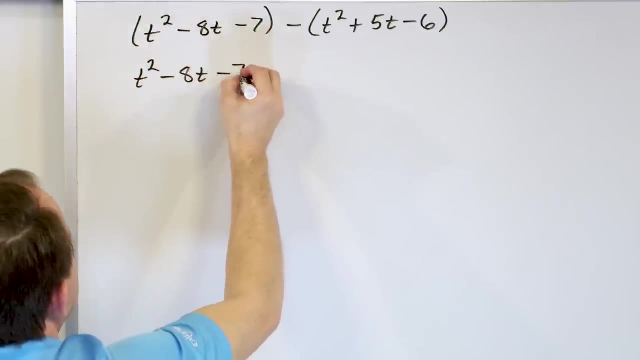 drop the parentheses is if you distribute the negative one in multiplying times every term, The first term is unaffected. So it's going to be t squared minus eight times t minus seven, Negative one times. this gives you negative t squared Negative one times. this gives you: 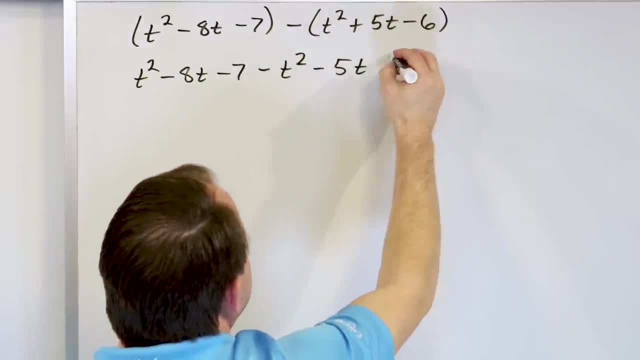 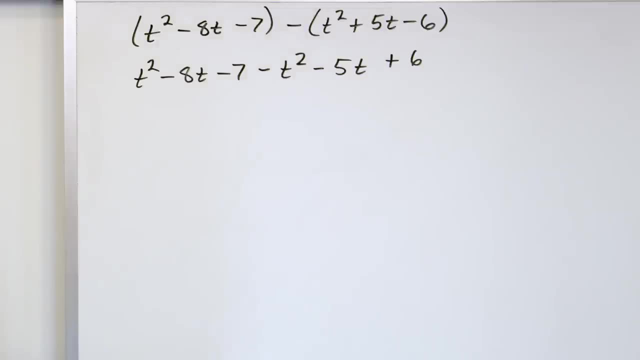 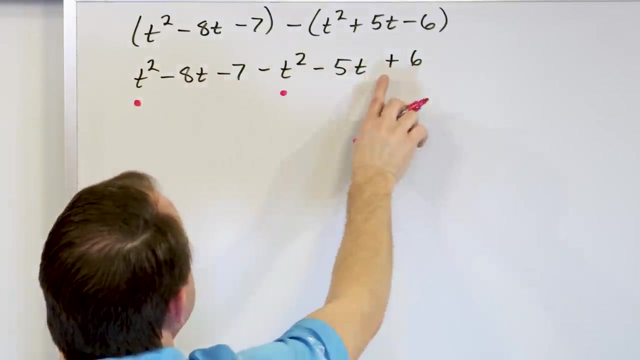 negative. five times t Negative. one times negative: six gives you a positive six. Don't forget that positive because of the multiplication here I'm going to start looking at what I can add together. I have a t squared term here. I keep going. I have another t squared term here. I don't have any other t squareds, So I have a positive one. 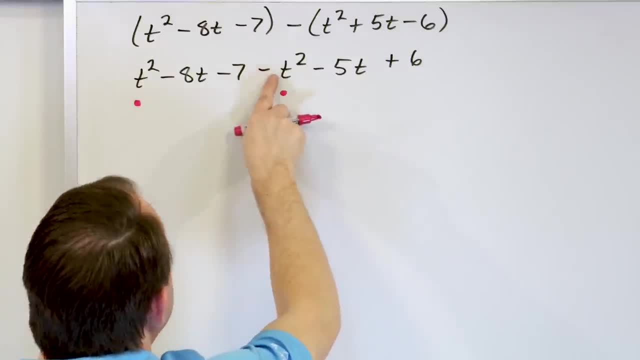 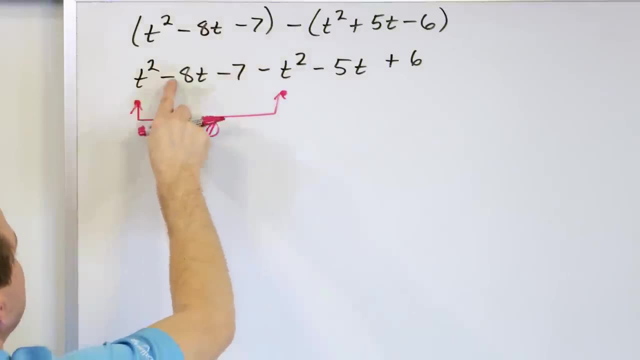 minus one, So positive one plus a minus one, Or you can think of it as one minus one. So really, what's going to happen with these terms? it's going to give you zero. The t squares are going to disappear because it's one minus one. So they're going to disappear, And just to have 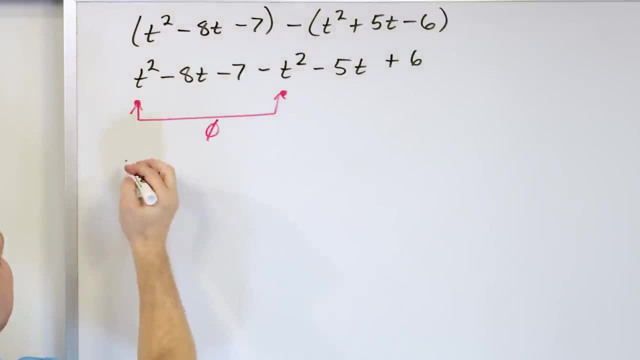 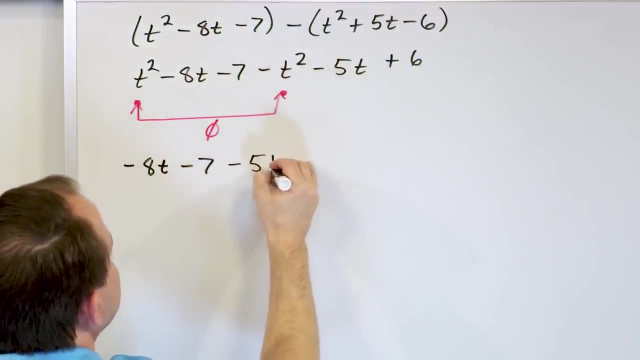 absolute clarity. I'm going to rewrite everything that's left over. This is left over. This is left over. You're going to have negative eight t minus seven. The t squared's gone. Now we have minus five t plus six, So the t squareds are gone. That's all I've done. And now I 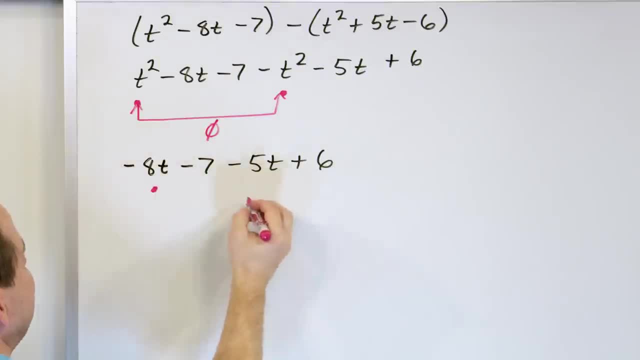 look and see. Here's a term with t. Here's a term with t. What is negative eight minus five? Or think of it as negative eight plus a negative five. Then what you're going to get there is it's going to be a 13, negative 13 times t. Then I have the negative seven. 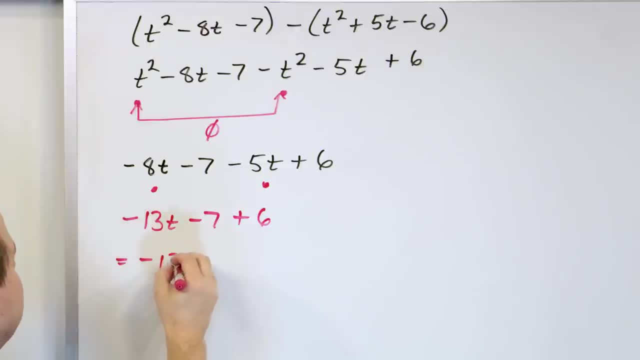 Then I have the positive six, And then I can add those Negative 13.. What is negative? seven plus six, You're going to get negative one. So negative 13 minus one. Negative 13 t. I should say Almost made a mistake there. 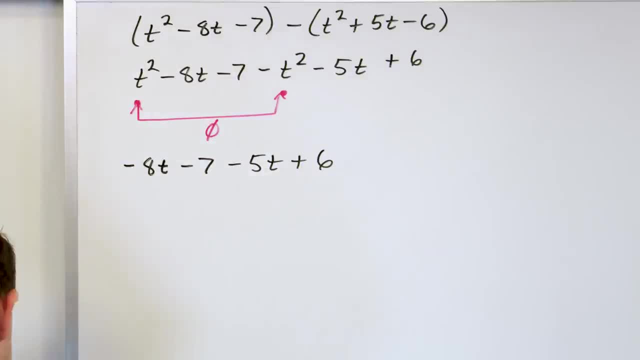 So the t squareds are gone. That's all I've done. And now I look and see: Here's a term with t, Here's a term with t. What is negative? eight minus five, Or think of it as negative eight plus a negative five. 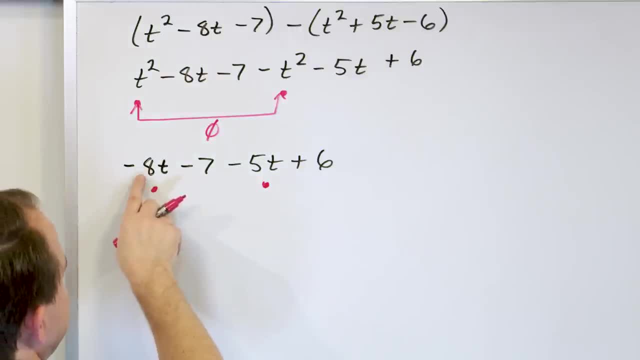 Then what you're going to get there is it's going to be a 13. Negative 13 times t, Then I have the negative seven, Then I have the positive six, And then I can add those Negative 13.. What is negative? seven plus six? 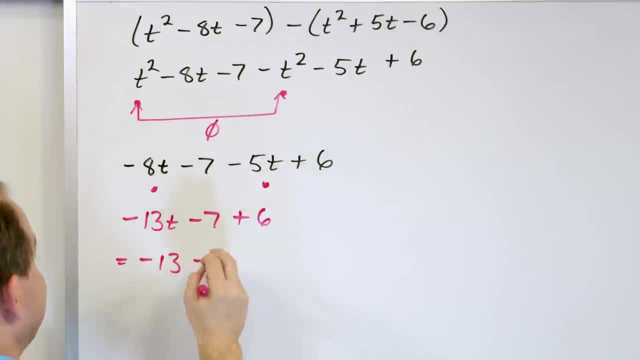 You're going to get negative one. So negative 13 minus one Negative 13t. I should say Almost made a mistake there. So here's negative 13t. Then you have this guy which is going to give you minus one. 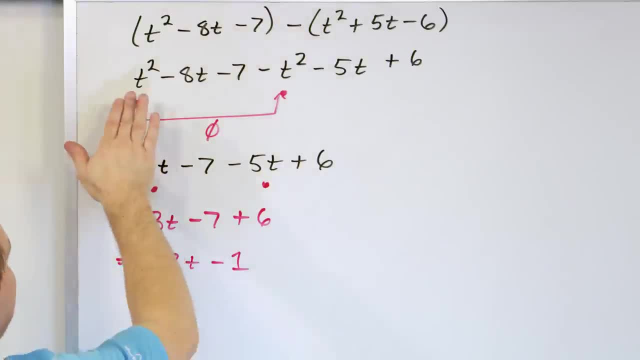 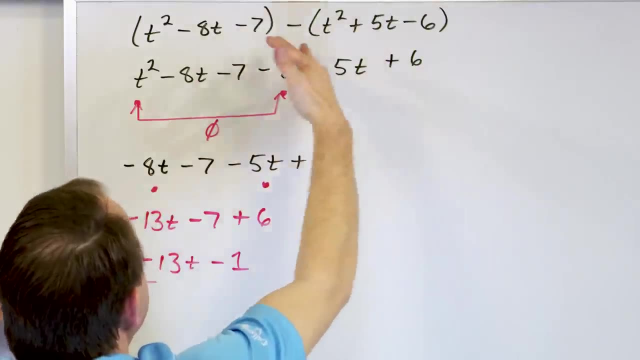 This is the final answer to the problem. So sometimes that happens. Sometimes variables disappear. If you have the same coefficient with different signs, it's going to drop away, And even though they are present in the original polynomial, when you add it all together and simplify it, 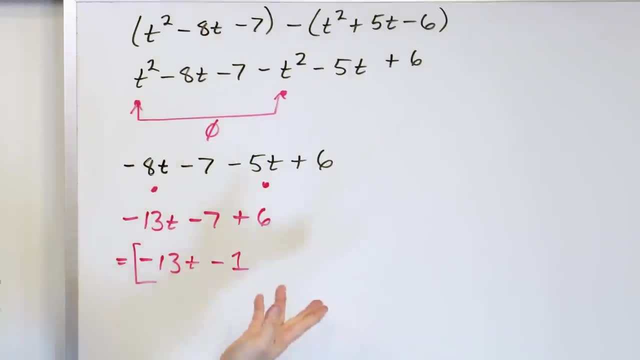 this is going to not have the t squared terms at all And I'll just take this time for a slight aside. This guy here, this negative 13t plus one, mathematically is exactly the same thing as this big thing up here. 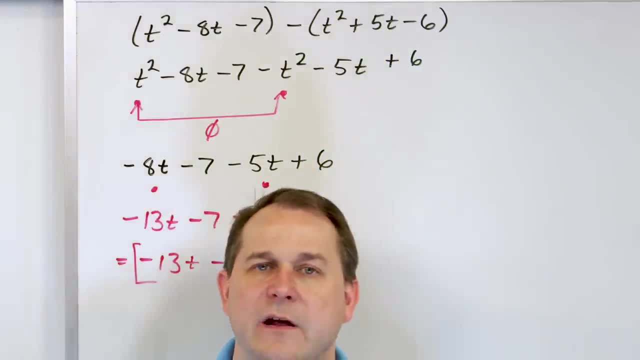 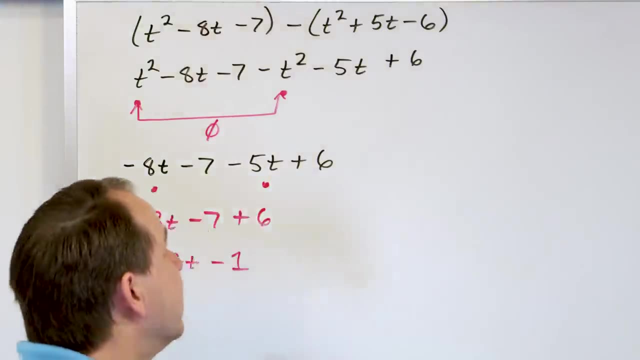 Because they're all equal. as you go down, You know, just like with fractions, You know 50 over 100 is the same as one half. They look different but they're very much exactly the same thing. This large term subtracted with this large term. 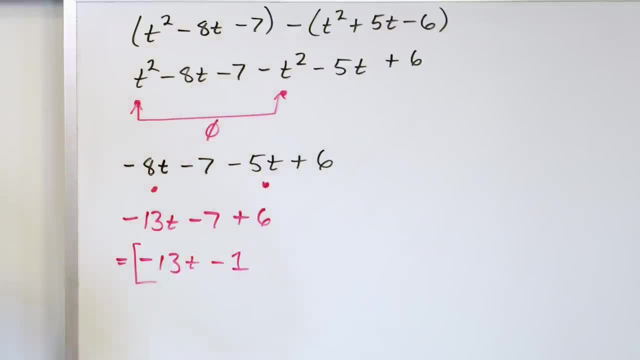 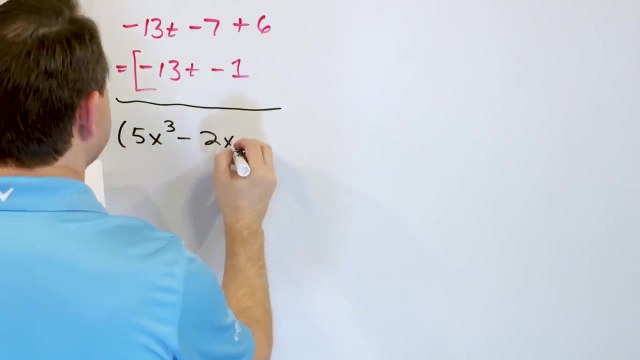 is exactly the same thing as this. So when we say simplify, we mean get rid of all the terms and simplify and tidy up everything you can by combining like terms: Negative, 13t minus one. Now the next one. let's say we have 5x to the third minus 2x plus one. 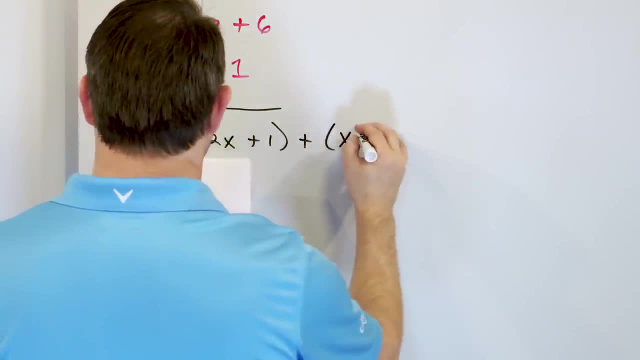 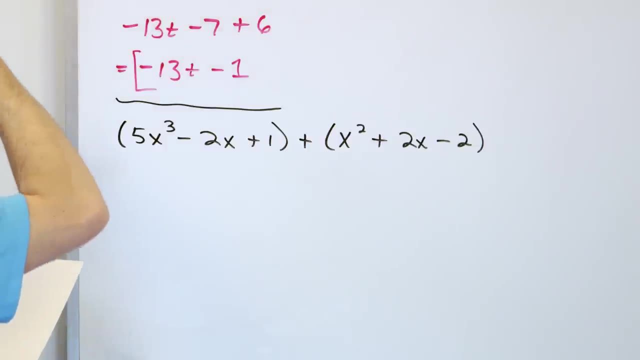 And we're going to add that to x squared plus 2x minus two. Let me just double check: 5x squared minus 2x plus one. x squared plus 2x minus two, Because it's just a plus one here. 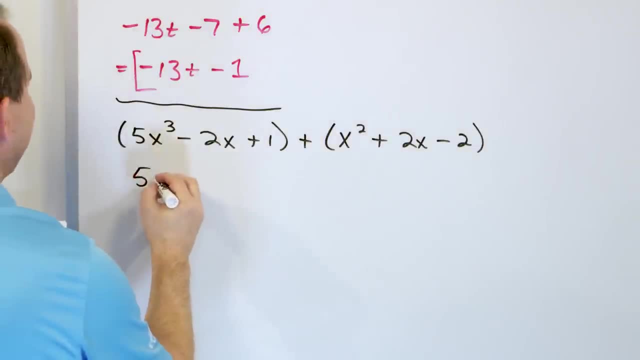 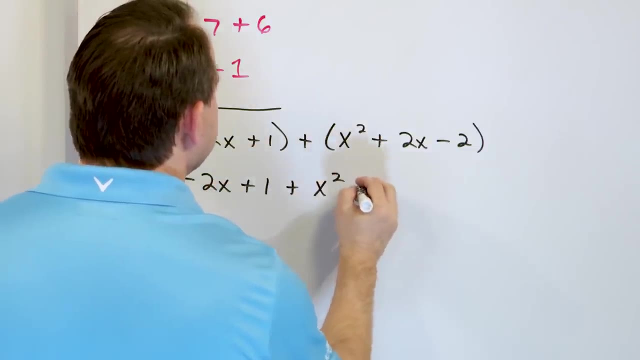 you're going to distribute it in, but it's not going to actually do anything. So we can just write everything without the parentheses entirely. 5x cubed minus 2x plus one. Then we'll just add the x squared plus the 2x minus the two. 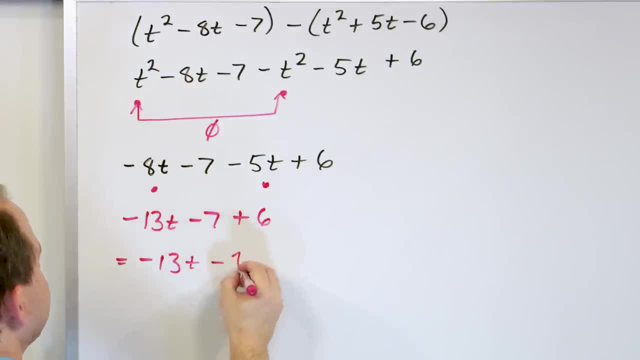 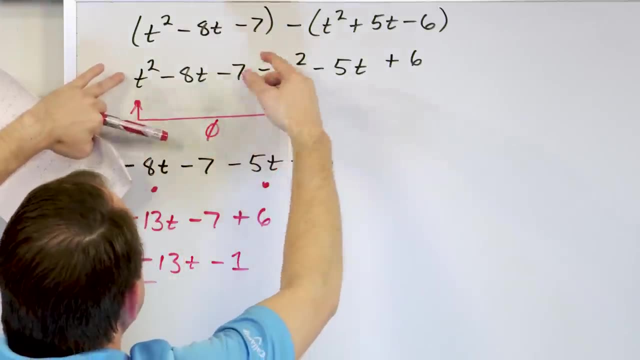 So here's negative 13 t. Then you have this guy which is going to give you minus one. This is the final answer to the problem. So sometimes that happens. Sometimes variables disappear. If you have the same coefficient with different signs, it's going to drop away. 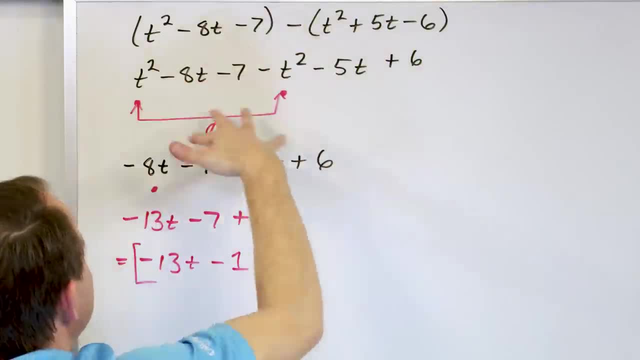 And even though they are present in the original polynomial, when you add it all together and simplify it, this is going to not have the t squared terms at all, And I'll just take this time for a slight aside. This guy here, this negative 13 t plus one. 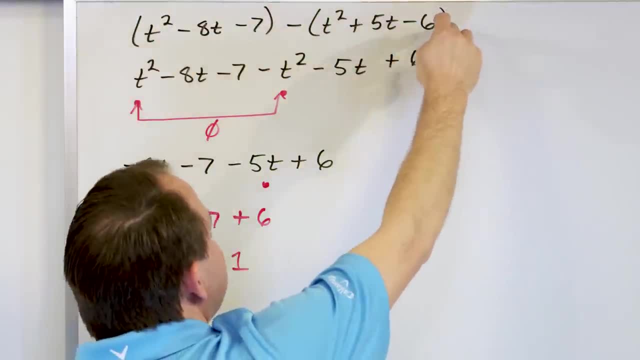 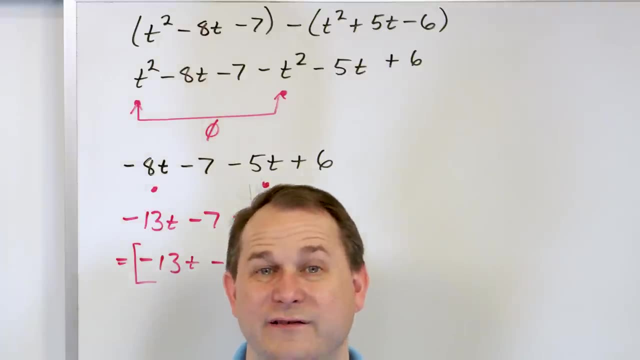 mathematically is exactly the same thing as this big thing up here, Because they're all equal as you go down, Just like with fractions: 50 over 100 is the same as one half. They look different, but they're very much exactly the same thing. This large term subtracted with this large term. 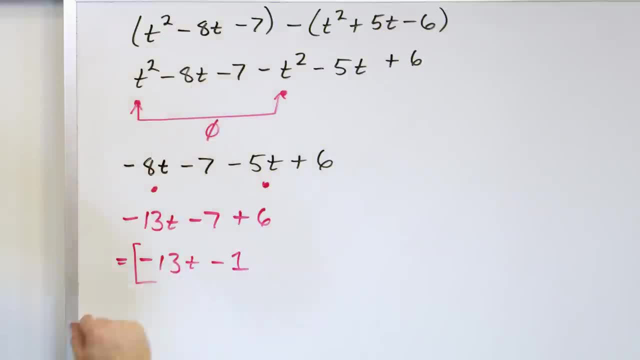 is exactly the same thing as this. So when we say simplify, we mean get rid of all the terms and simplify and tidy up everything you can, And then we're going to get rid of all the terms, And then we're going to get rid of all the terms and simplify everything you can by combining like terms. 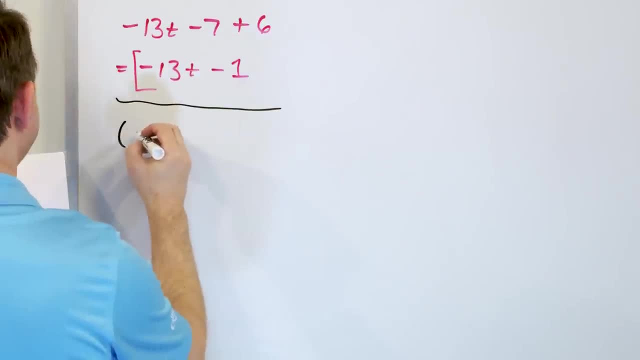 Negative: 13t minus one. Now the next one. let's say we have five x to the third minus two x plus one, And we're going to add that to x squared Plus two X minus two. Let me just double check: Five x squared minus two x plus one, x squared plus two X minus two. 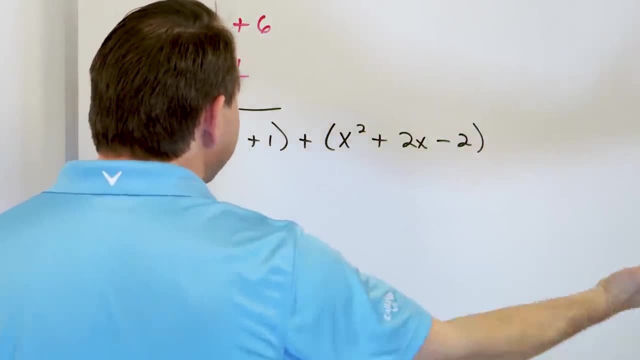 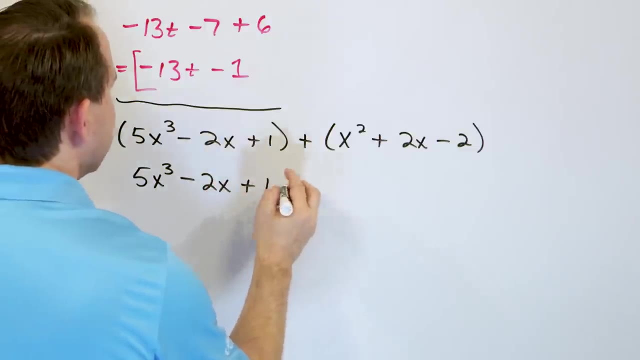 Now, because it's just a plus one here and you can distribute it in, but it's not going to actually do anything. So we can just write everything without the parentheses. parentheses entirely: 5x cubed minus 2x plus 1. then we'll just add the x squared plus the 2x. 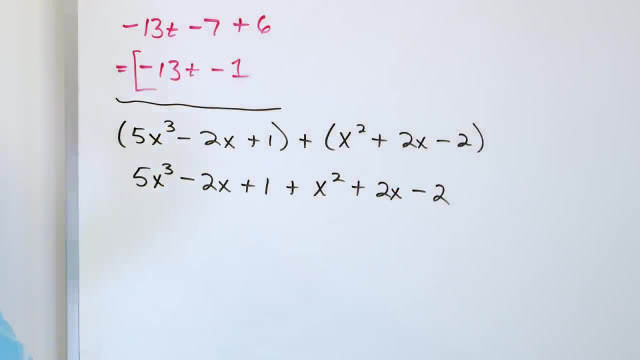 minus the 2, and then we'll look for like terms. we look for the biggest value of power of x, first x cubed, and we don't have any other x cubed anywhere else, so we'll just write the first term down as 5x cubed. then we look for powers of x squared. we see we have an x squared here, but 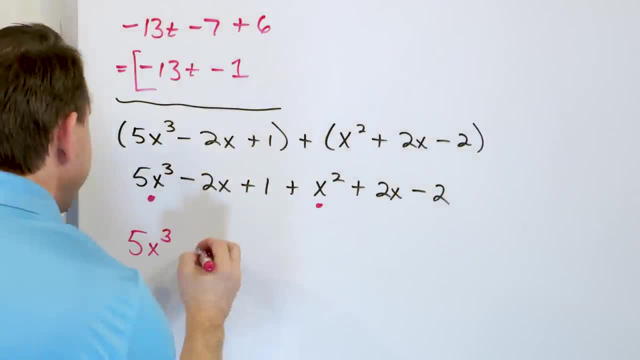 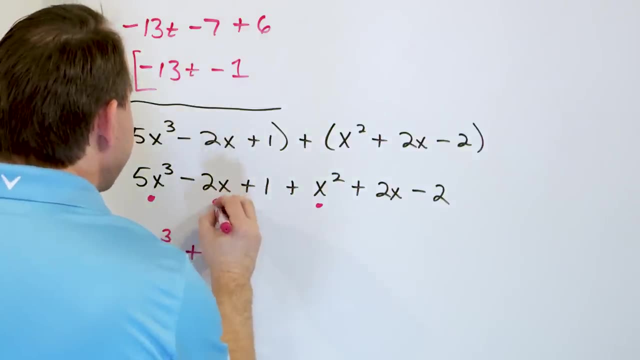 again, there's only one of them and there's no other x squareds anywhere there. so again, we just write x squared down. so so far i haven't had to actually do anything. now i look at this: i have a negative 2x and a positive 2x. so when you actually add these two things together, negative 2 plus a. 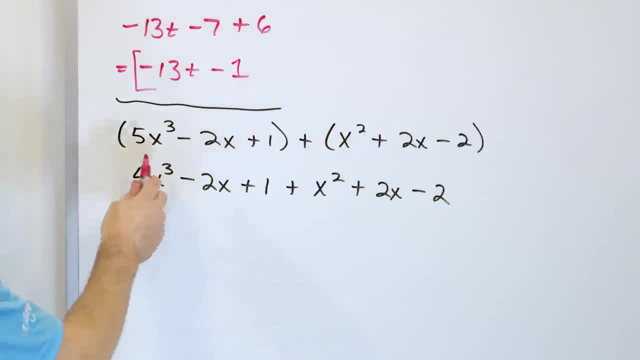 And then we'll look for like terms. We look for the biggest value of power of x, first x cubed, And we don't have any other x cubed anywhere else, So we'll just write the first term down as 5x cubed. 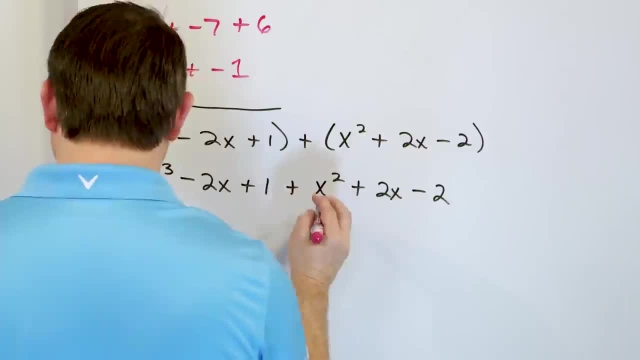 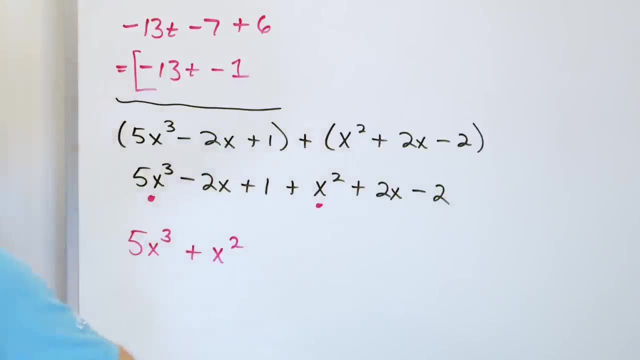 Then we look for powers of x squared. We see we have an x squared here, but again there's only one of them And there's no other x squared anywhere there. So again we just write x squared down. So so far I haven't had to actually do anything. 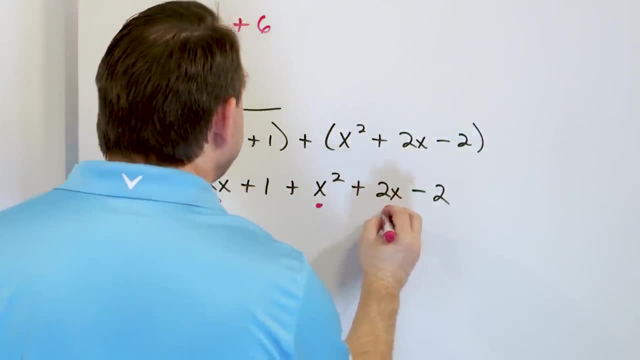 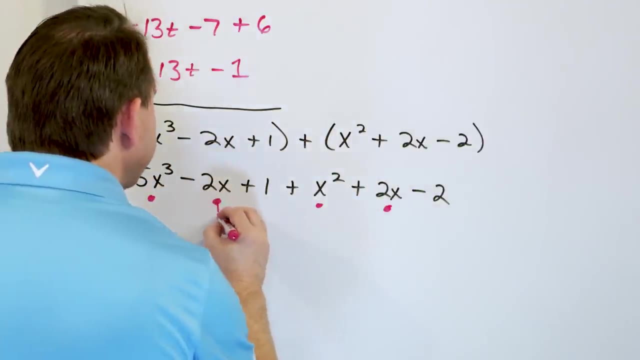 Now I look at this, I have a negative 2x and a positive 2x. So when you actually add these two things together- negative two plus a positive two- you're actually going to get zero. So I'll just kind of show you that by connecting these guys. 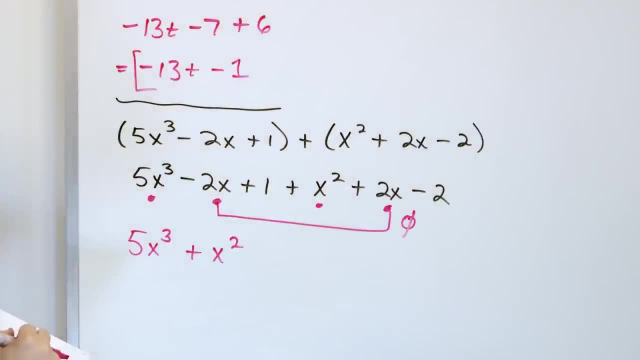 and putting a zero to remind you that these add, to give you zero. And then you're just going to look at the numbers: One minus two. What is one minus two? It's negative one, So you can actually add this together. So the answer that you're going to get is 5x cubed plus x squared minus one. 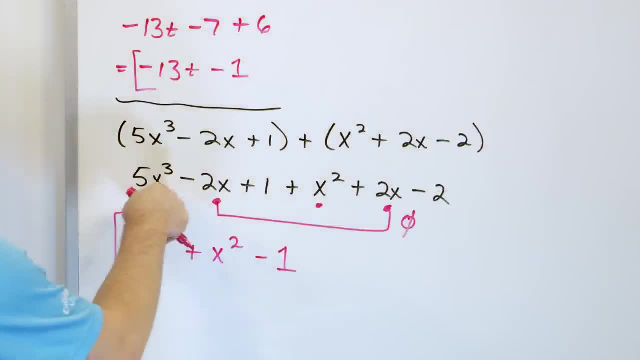 That's the final answer. So we drop the parentheses. We can't add anything to this, so it comes down. We can't add anything to this, so it comes down. We try to add these, but it gives us zero, so it drops away. 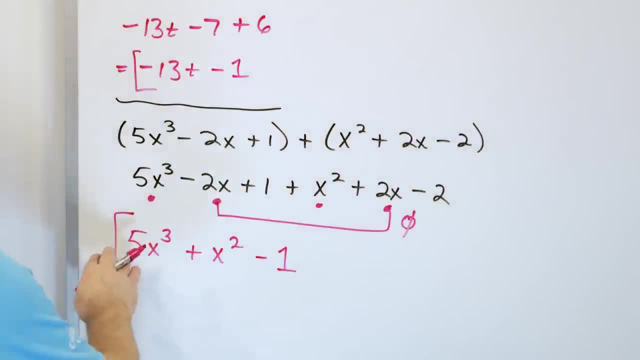 And then one minus two gives us the negative one, And this is in decreasing powers of x. And again as a bonus question: what type of polynomial is this? It's got one, two, three terms, so we call it a trinomial. 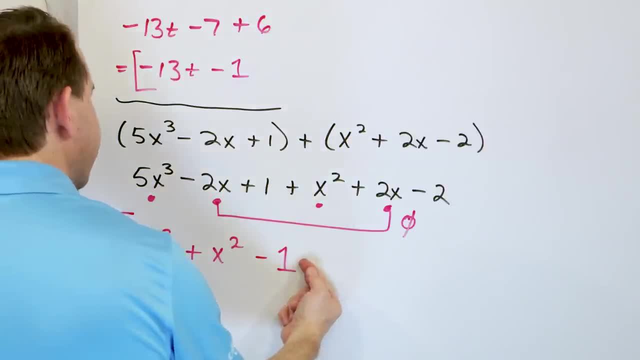 And what is the degree of this polynomial? Well, the degree of this term is zero. The degree of this term is two. The degree of this term is three. So the degree of the whole thing is three, the largest degree of everything listed. 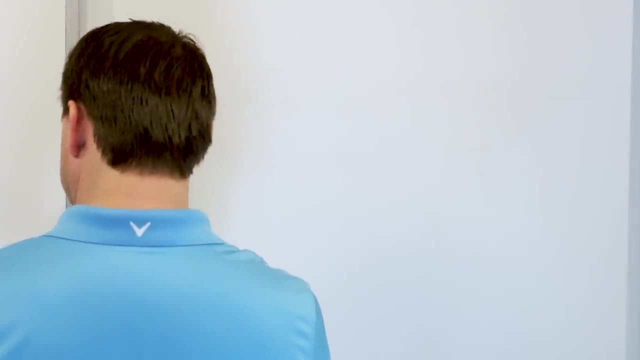 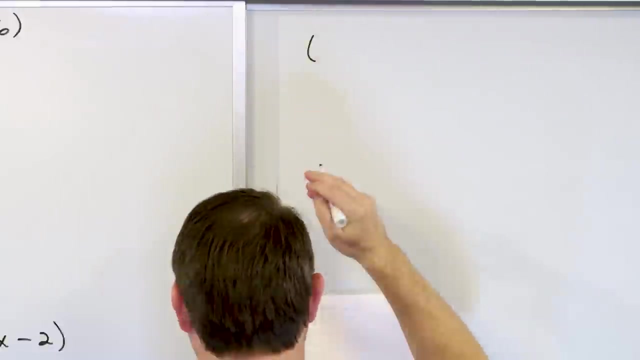 All right, Now let's do the next one. We only have a few more of these guys, But they're all really, really important. What if we have Notice? what we're going to do here is: I've taken these and added them together. 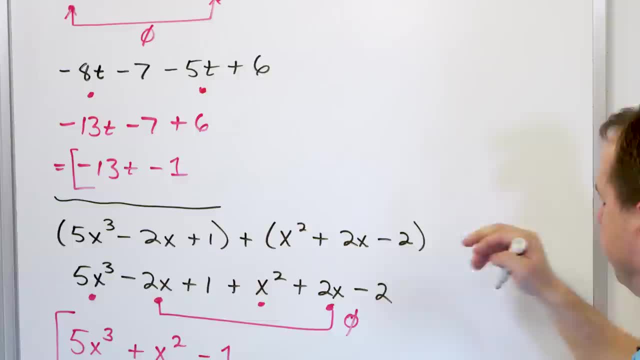 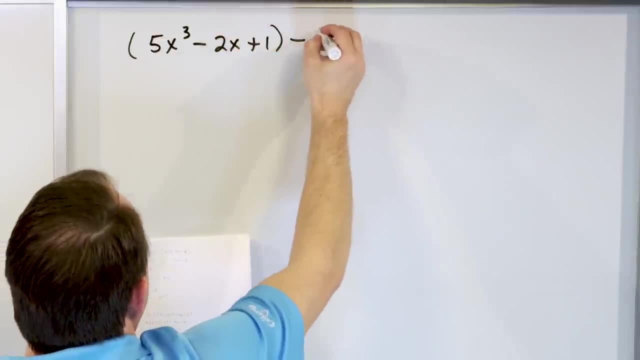 And the next problem: we're going to take these two polynomials and just subtract them. So that's the only difference between them. So that's the only difference between these problems: Five x cubed minus two x plus one. Close it off. 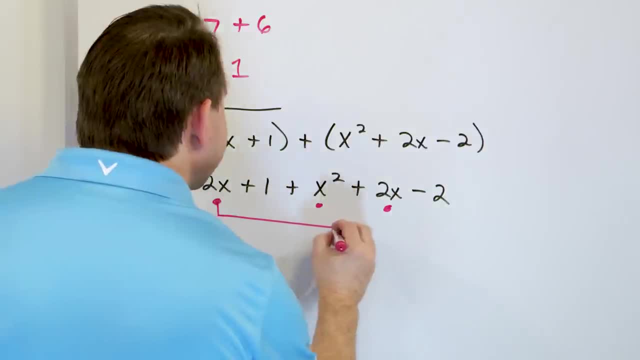 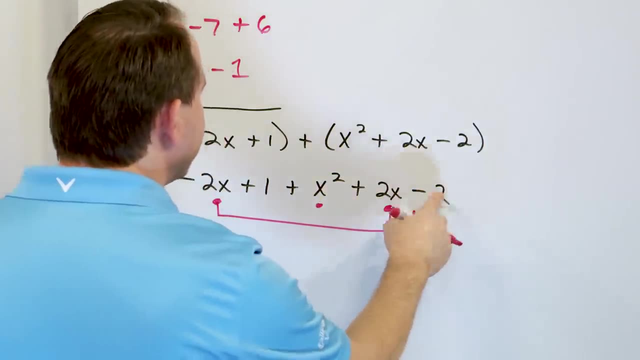 positive 2, you're actually going to get zero. so i'll just kind of show you that by connecting these guys and putting a zero to remind you that these add, to give you zero, and then you're just going to look at the numbers: 1 minus 2. what is 1 minus 2? it's negative 1, so you can actually add. 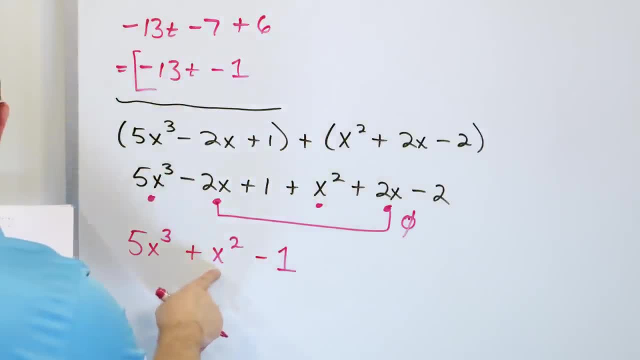 this together, so the answer that you're going to get is 5x cubed plus x squared minus 1. that's the final answer, so we drop the parentheses. we can't add anything to this, so it comes down. we can't add anything to this, so it comes down. we try to add these, but it gives us. 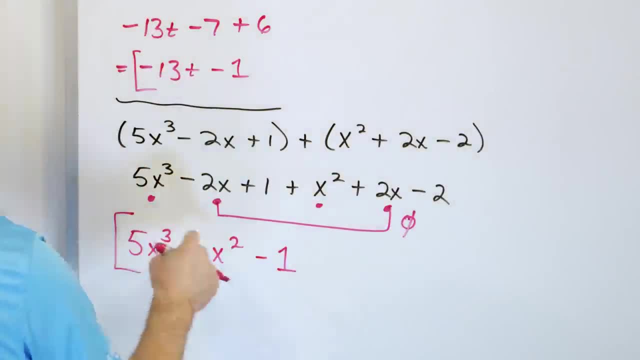 zero, so it drops away, and then 1 minus 2 gives us the negative 1, and this is in decreasing powers of x. and again, as a bonus question: uh, what type of polynomial is this? it's got one, two, three terms. we call it a trinomial. and what is the degree of this polynomial? well, the degree of this term is: 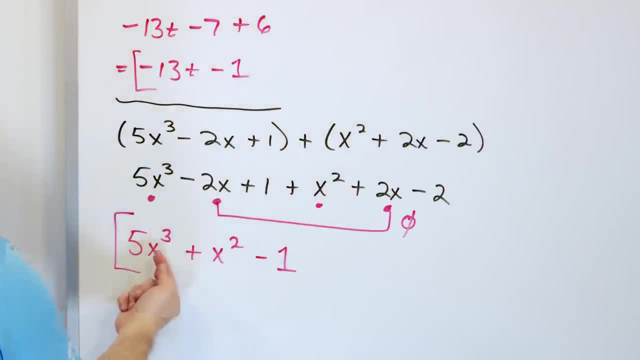 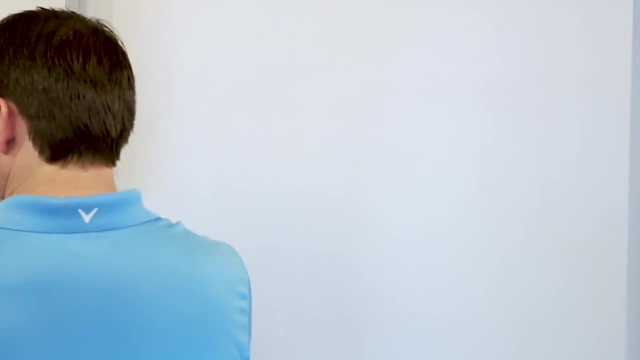 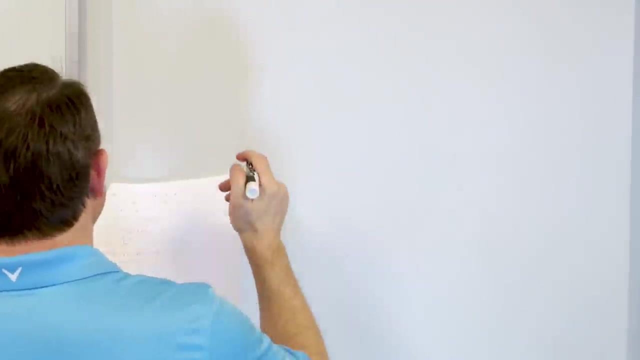 zero. the degree of this term is two. the degree of this term is three, so the degree of the whole thing is three, the largest degree of everything listed. all right, now let's do the next one. we only have a few more of these guys, but they're all really, really important. what if we have um? notice? what we're going to do here is i've 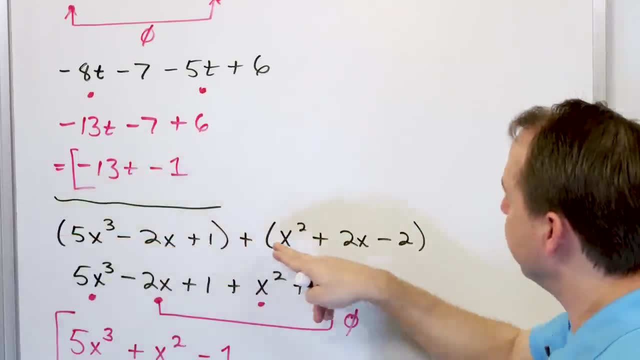 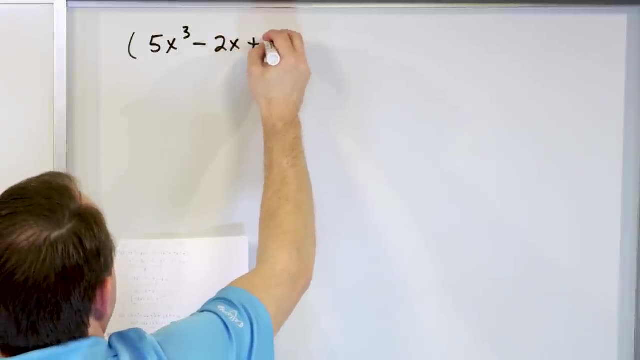 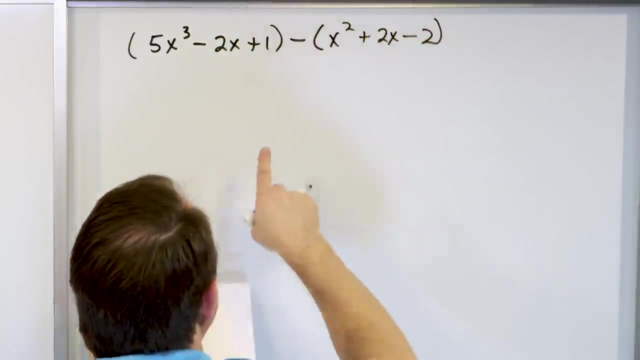 taken these and added them together. and the next problem: we're going to take these two polynomials and just subtract them. so that's the only difference between these problems: 5x cubed minus 2x plus 1. close it off. open the next one: x squared plus 2x minus 2.. this problem is exactly the same as the. 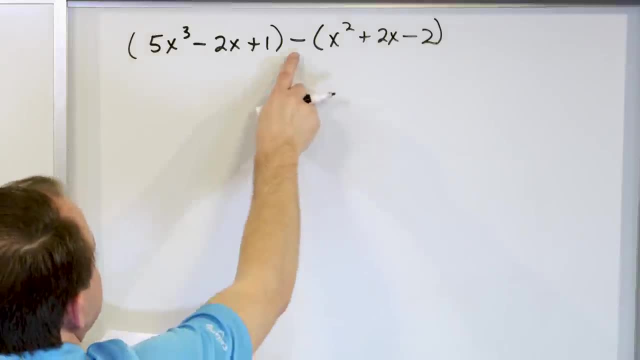 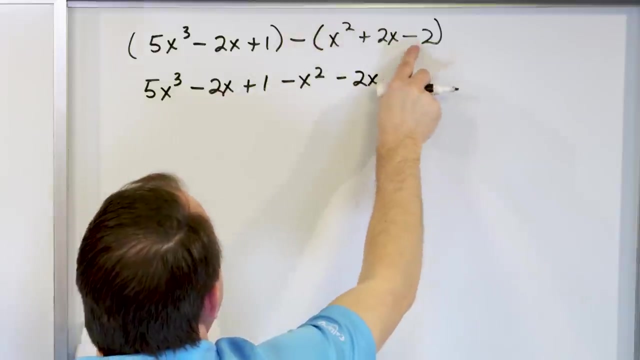 previous, except now i have a minus sign there, which means that i need to distribute the negative 1 in so i can add things together. so i have 5x cubed minus 2x plus 1 negative 1 times. this is negative. x squared negative 1 times. this is negative. 2x. negative 1 times. this is positive 2. 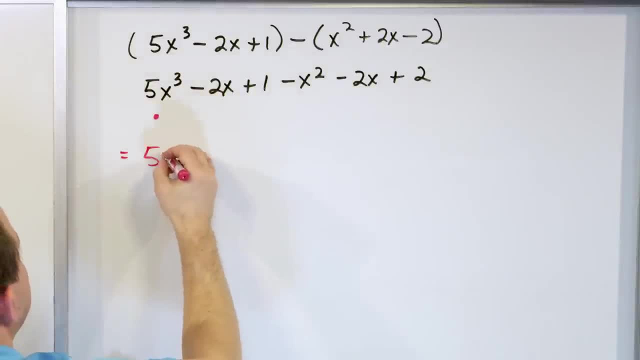 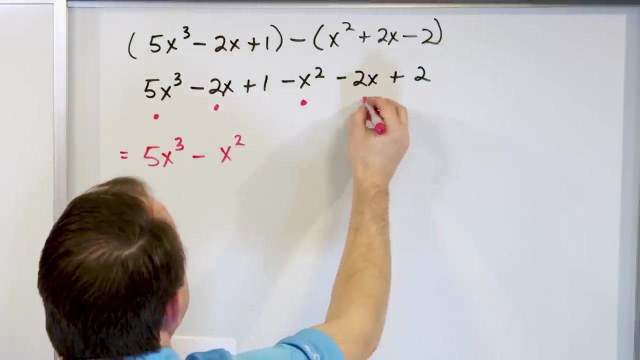 there are no other x cubed terms, so 5x cubed comes along for the ride. then i look for x squared. here's an x squared, but there's no other x squared terms anywhere, so i carry it along as negative x squared right. then i look at x terms. here's a term, here's a term. negative 2, negative 2. i add them together. 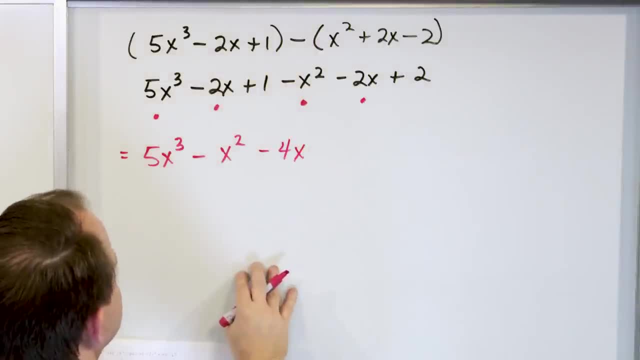 negative 2 plus negative 2 is negative 4 times x and just for clarity, i'll drag the 1 down here and i'll drag the 2 down here, but i'll add those in the next step. even though it's kind of simple, i don't really have to do that. 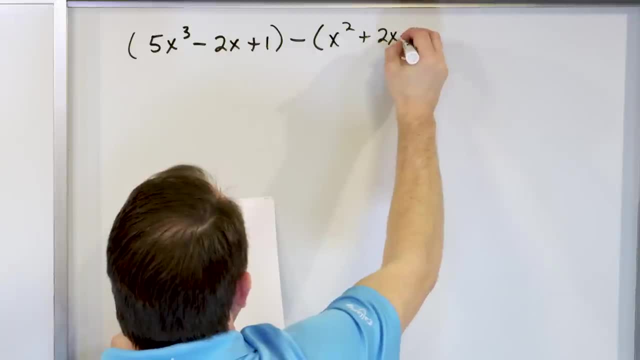 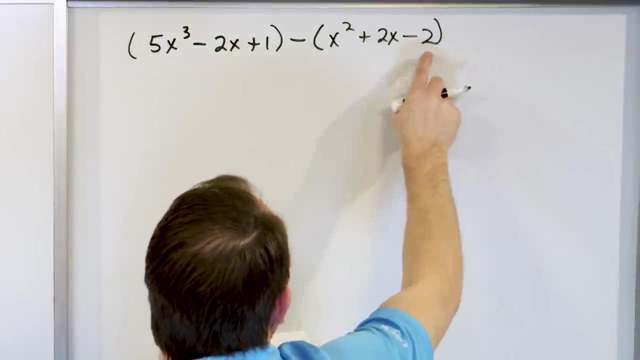 Open the next one: X squared plus two x minus two. This problem is exactly the same as the previous, except now I have a minus sign there, which means that I need to distribute the negative one in, so I can add things together. So I have five x cubed minus two x plus one. 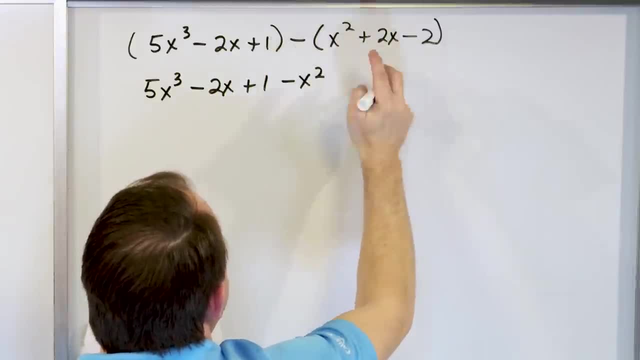 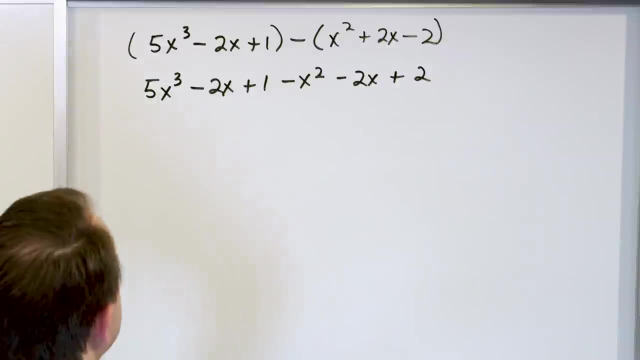 Negative. one times this is negative. x squared Negative. one times this is negative. two x Negative. one times this is positive two. Then I start looking for things to add together Again: five x cubed. There are no other x cubed terms. 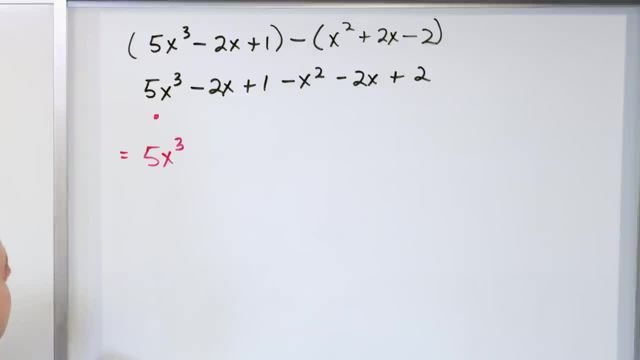 So five x cubed comes along for the ride. Then I look for x squared. Here's an x squared, But there's no other x squared terms anywhere, So I carry it along as negative x squared Right. Then I look at x terms. 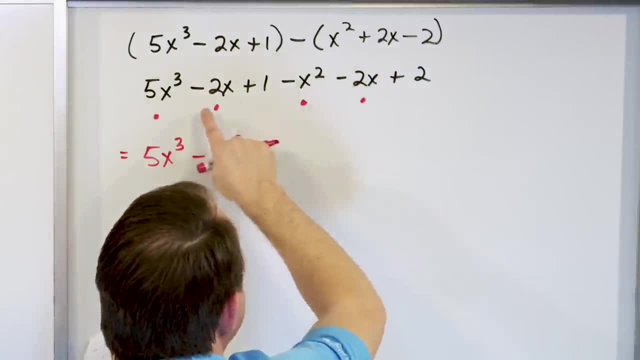 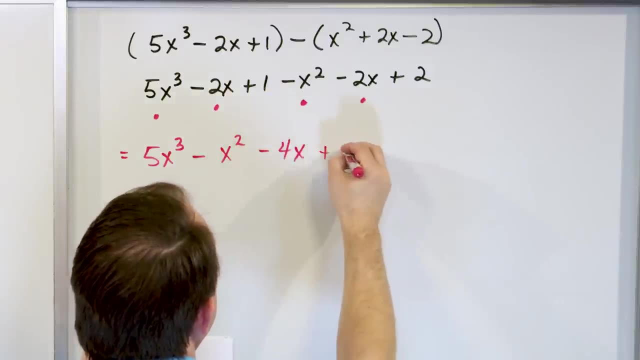 Here's a term. Here's a term: Negative two, Negative two. I add them together. Negative two is negative four times x And just for clarity, I'll drag the one down here and I'll drag the two down here, But I'll add those in the next step, even though it's kind of simple. 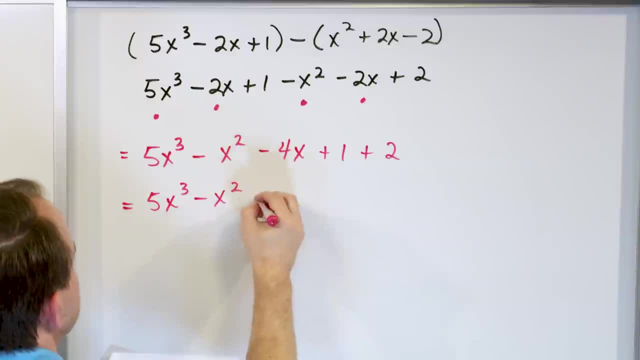 I don't really have to do that. Five x cubed minus x, squared minus four x, And then this becomes a plus three. Let me double check: Five x cubed minus x, squared minus four x plus three. So this is the final answer. 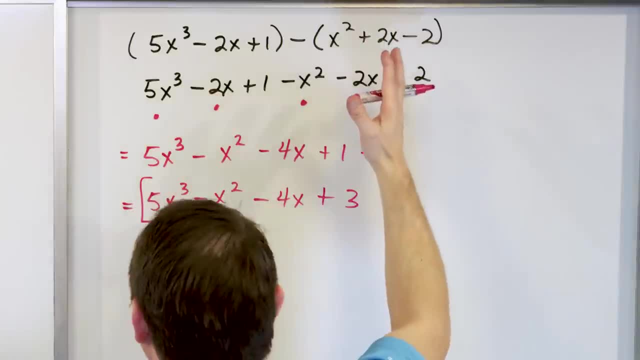 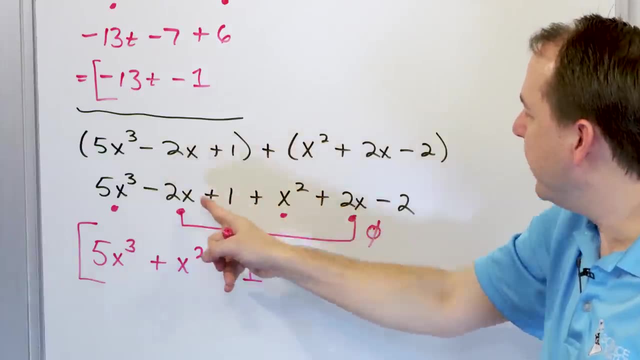 Correct, And this problem is exactly the same as the previous one. It's just one was added and one was subtracted. It made all the difference in the world Because when they were added together, that caused these terms to kill each other, and 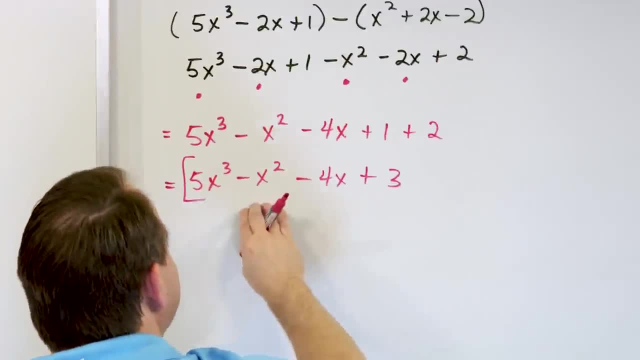 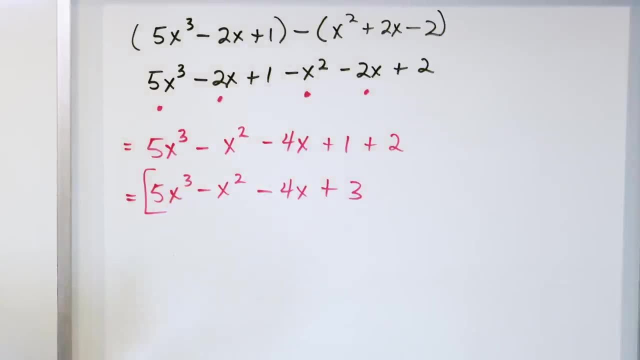 basically annihilate and give you zero, And that didn't happen here, And that's why we have more terms. This is a polynomial, again, of degree three, The highest degree of all the terms that are present. I only have two more problems. 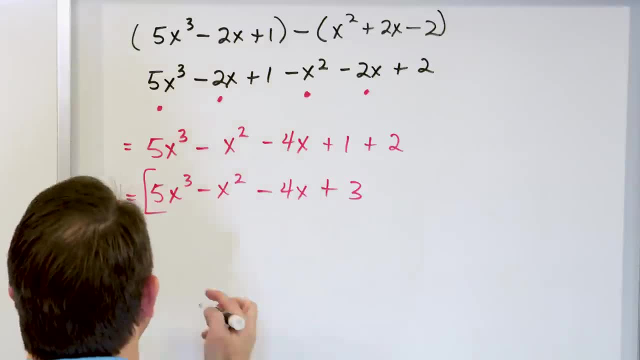 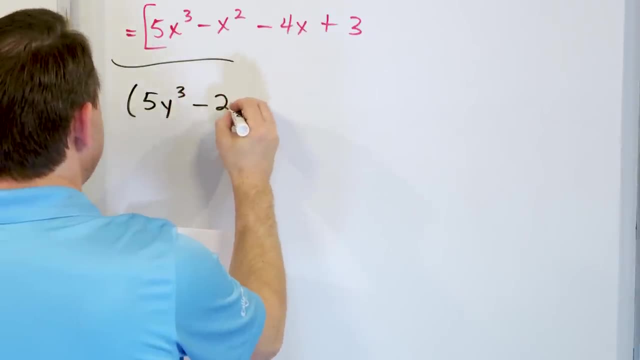 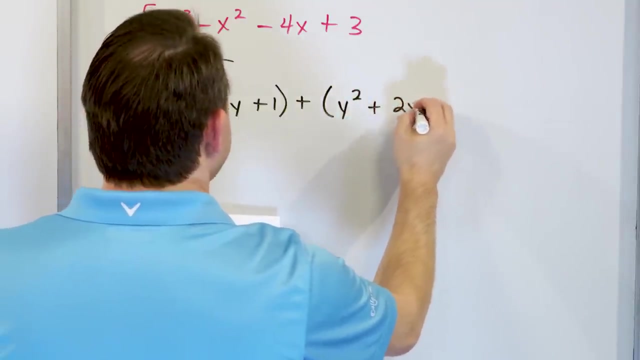 One that we will do on this board and one that we will do on the next one. So what if we have five times y cubed minus two times y plus one And we'll add that to y squared plus two y minus two? Let me just double check. it's correct. 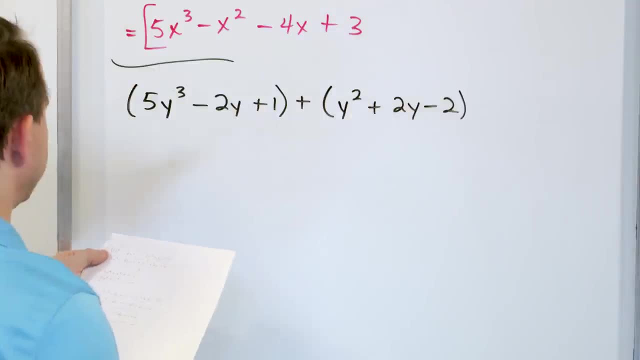 Five y cubed minus two y plus one, And then y squared plus two y minus two. It's a plus sign, So I'm distributing a one and it's not going to change anything, So I'll just rewrite it: Five y cubed minus two y plus one, plus y squared plus two y minus two. 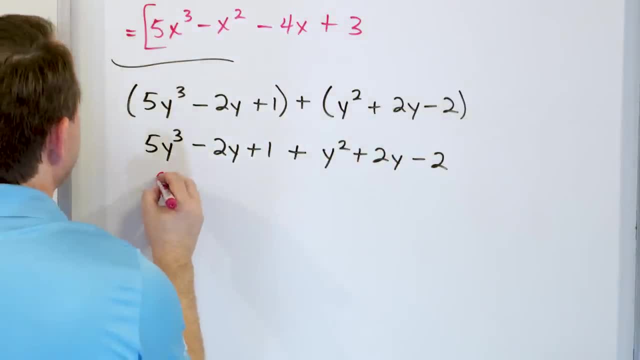 And then I start looking for things to add. Here's my largest power of y cubed. I don't have any other y cubed, So I'll just say five y cubed is my first term, Then I'll look for y squared. 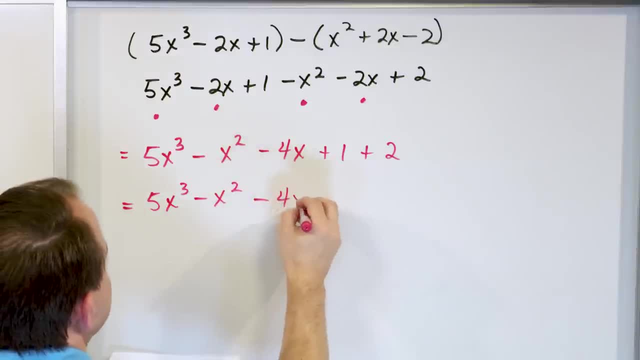 5x cubed minus x, squared minus 4x, and then this becomes a plus 3.. let me double check: 5x cubed minus x, squared minus 4x plus 3. so this is the final answer, correct, the only thing you have in. 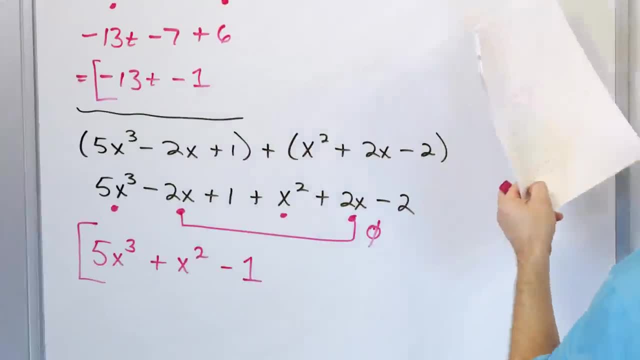 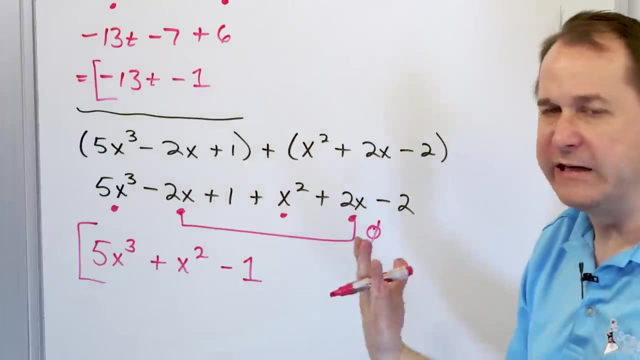 this problem is exactly the same as the previous one, it's just one was added and one was subtracted. it made all the difference in the world because when they were added together, that caused these terms to kill each other and basically annihilate, give you zero, and that didn't happen here. and 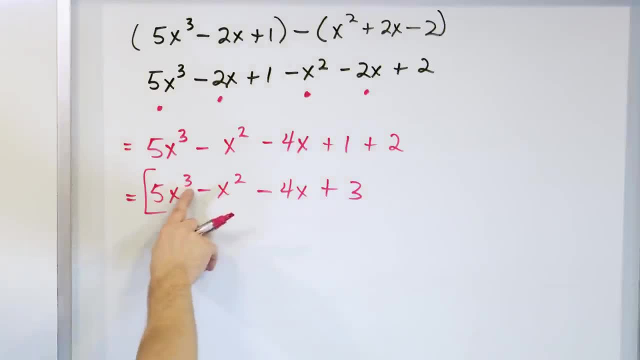 that's why we have more terms- this is the first one- is a polynomial, again, of degree 3, the highest degree of all the terms that are present. i only have two more problems, one that we will do on this board and one that we will do on the next one. 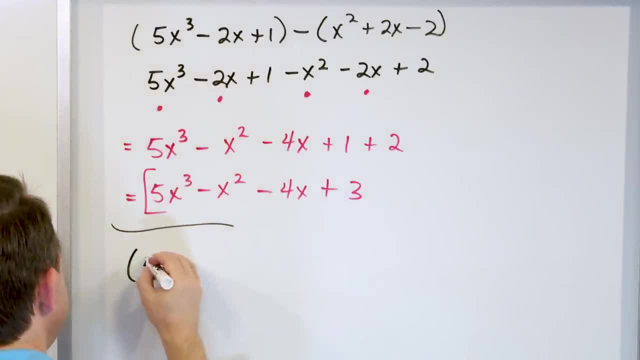 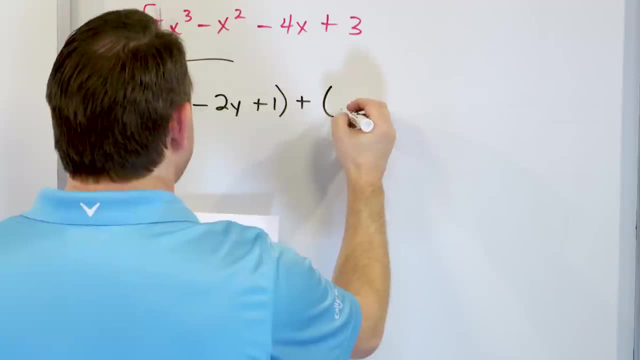 so what if we have 5 times y cubed minus 2 times y plus 1 and we'll add that to y squared plus 2i minus 2? let me just double check. it's correct: 5y cubed minus 2i plus 1. 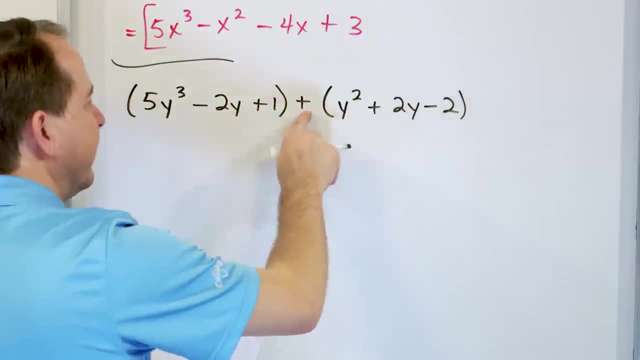 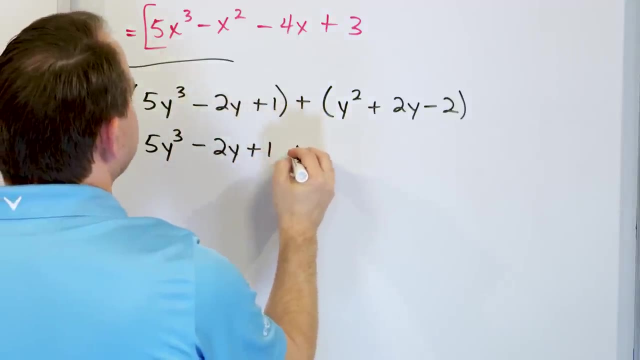 and then y squared plus 2i minus 2. it's a plus sign, so i'm distributing a 1 and it's not going to change anything, so i'll just rewrite it: 5y cubed minus 2y plus 1 plus y squared plus 2y. 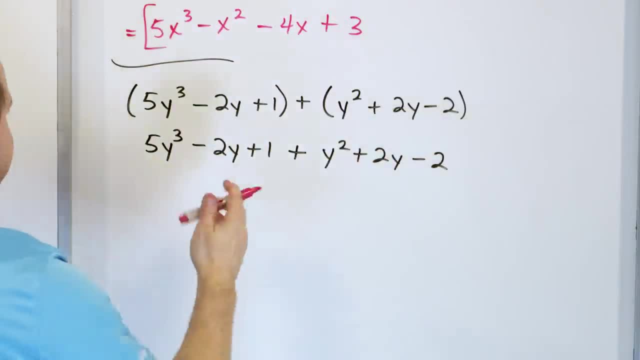 minus 2, and then i start looking for things to add. here's my largest power of y cubed. i don't have any other y cubes. so i'll just say 5y cubed is my first term, then i'll look for y squared. here's one. i don't have any other y square, it's anywhere. so the next term i don't. 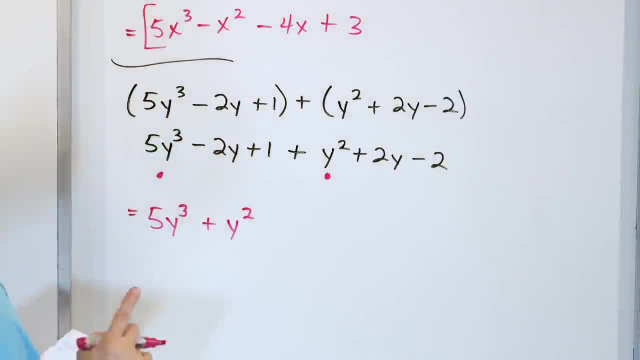 to really add it to anything. It's going to be y squared. Then again, I have a y term here and I look around and I have another y term here and it looks like the same thing happens. I have a negative 2 and I have a positive 2, just coincidence with the last. 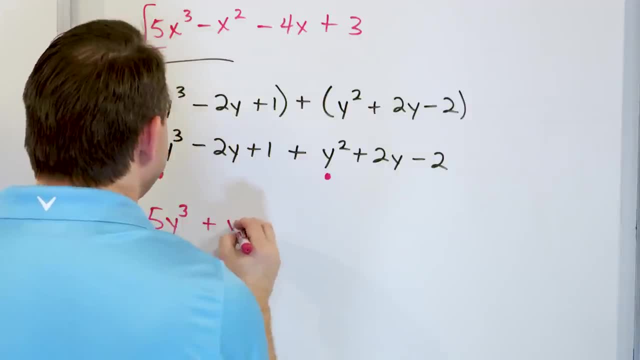 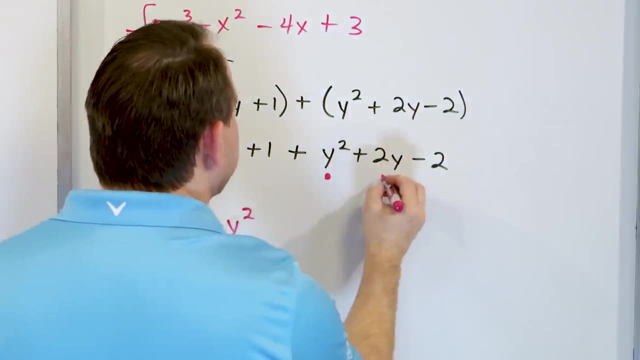 Here's one. I don't have any other y squared anywhere. So the next term I don't have to really add it to anything, It's going to be y squared. Then again, I have a y term here And I look around and I have another y term here. 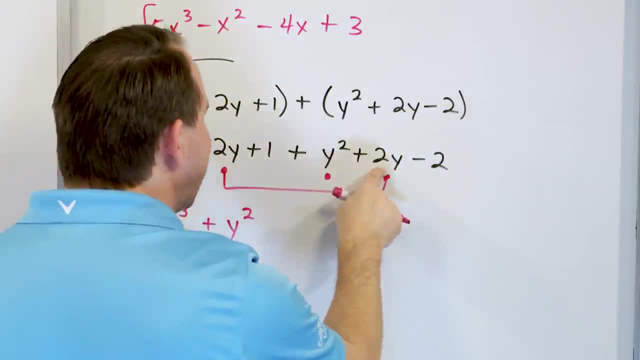 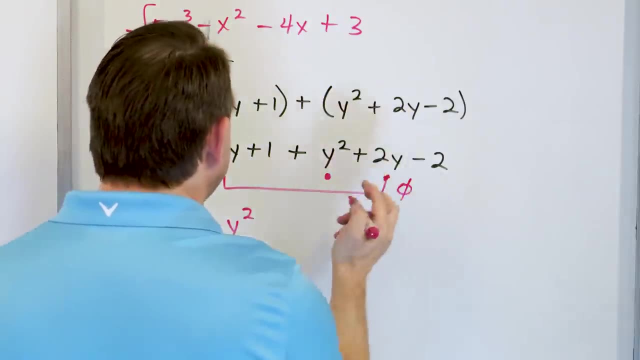 And it looks like the same thing happens. I have a negative two and I have a positive two- Just coincidence with the last problem- But they add to zero, so nothing happens, And then one minus two. I'll go ahead and write it like this: 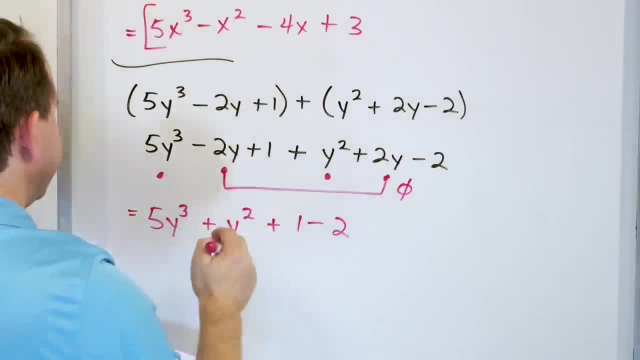 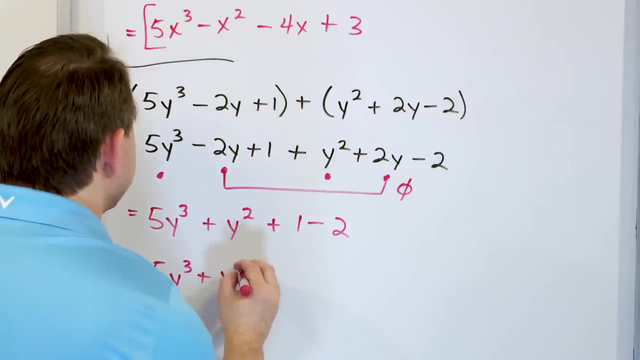 One minus two. So I'll have the plus one here, the minus two here. The y's kill each other and basically give you zero. So what I have is five times y cubed plus y squared. What is one minus two? It's negative one. 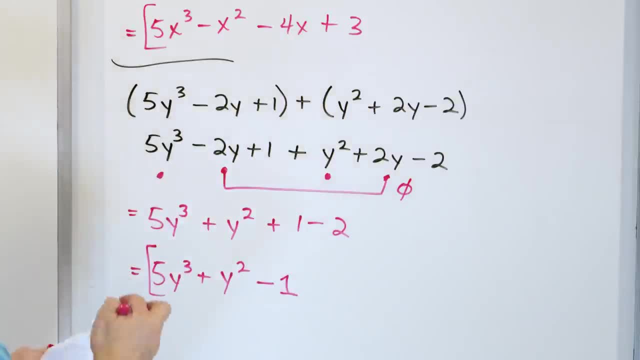 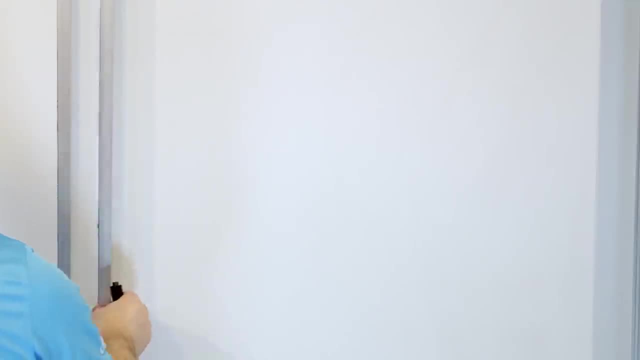 That's the final answer: Five y cubed plus y squared, minus one. Now on the final problem. we will take these exact same polynomials, but we'll have a minus sign in there. So we'll be subtracting the same polynomials instead of adding them. 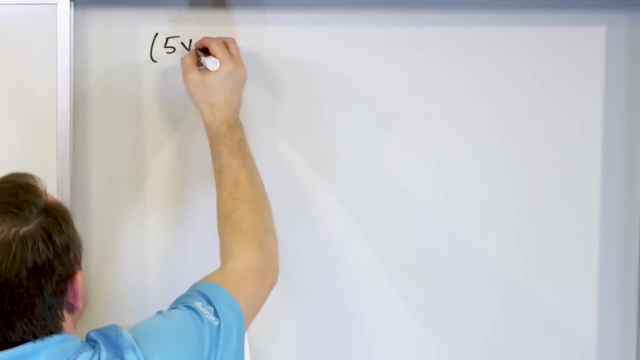 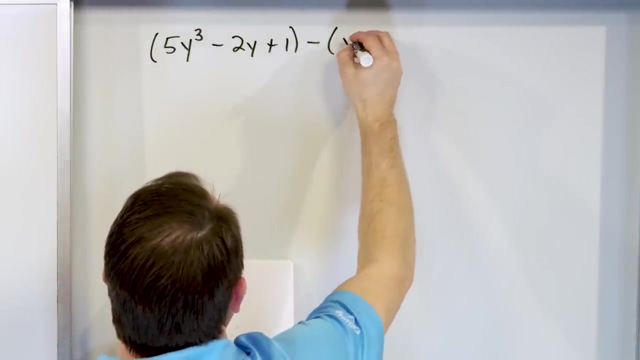 All right. So let's take a look. What if we have five y cubed minus two, y plus one, and we'll be subtracting the next term or the next polynomial trinomial, y squared plus two, y minus two, And we're going to subtract them. 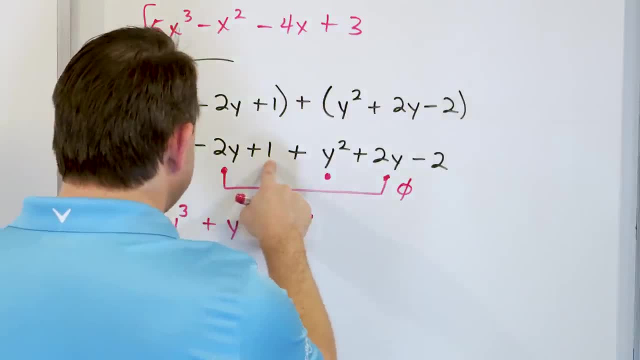 problem. but they add to 0, so nothing happens, And then 1 minus 2, I'll go ahead and write it like this: plus 1 minus 2.. So I'll have the plus 1 here, the minus 2, here the y's. 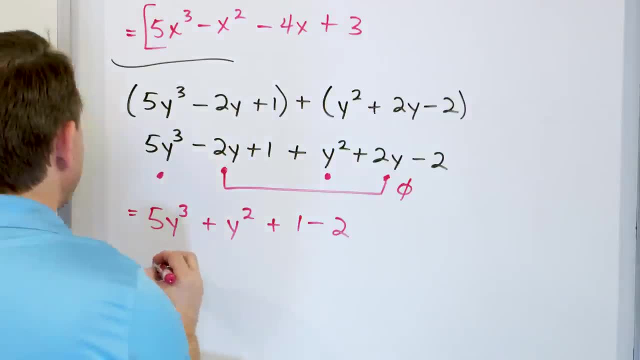 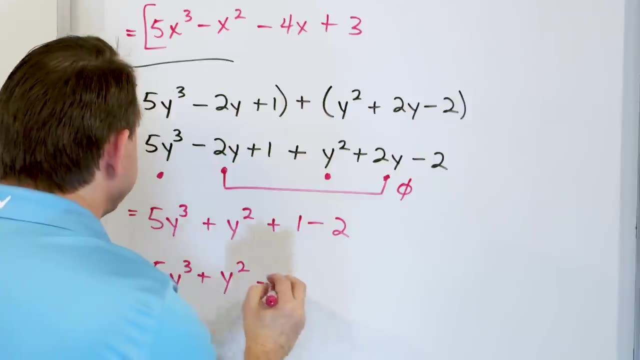 kill each other and basically give you 0.. So what I have is 5 times y cubed plus y squared. What is 1 minus 2?? It's negative 1.. That's the final answer: 5y cubed plus y squared. 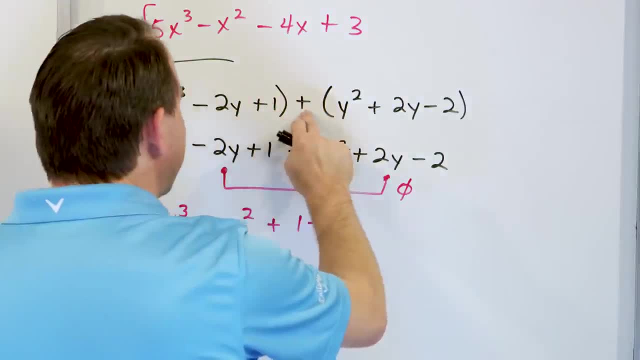 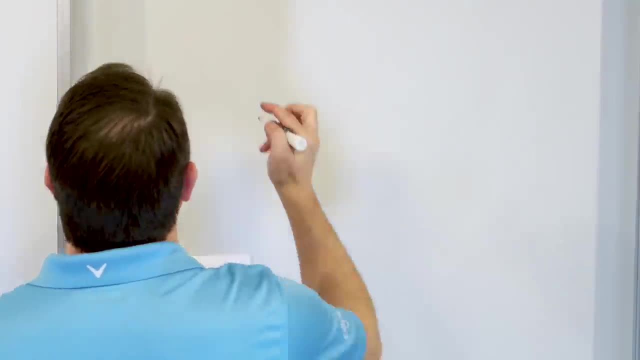 minus 1.. Now on the final problem. we will take these exact same polynomials, but we'll have a minus sign in there, So we'll be subtracting the same polynomials instead of adding them. So let's take a look: What if we have 5y cubed minus 2y plus 1 minus 2y squared plus? 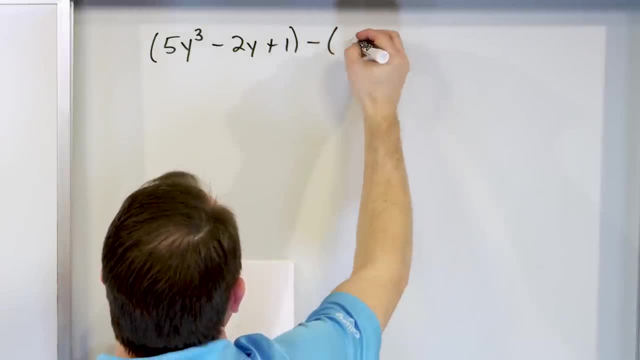 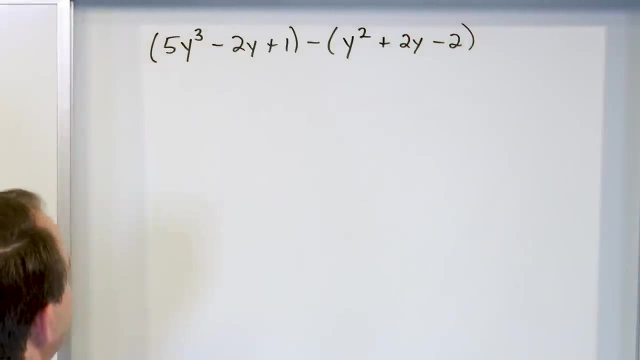 2y plus 1 and we'll be subtracting the next term or the next polynomial trinomial, y squared plus 2y minus 2.. And we're going to subtract them, which means we have to distribute this negative 1 in. So let's go ahead and do that: 5y cubed minus 2y plus 1.. What is? 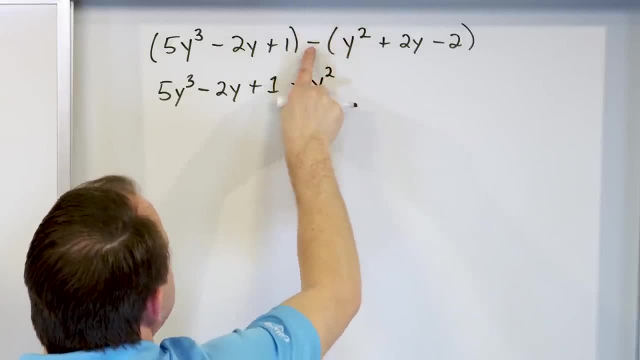 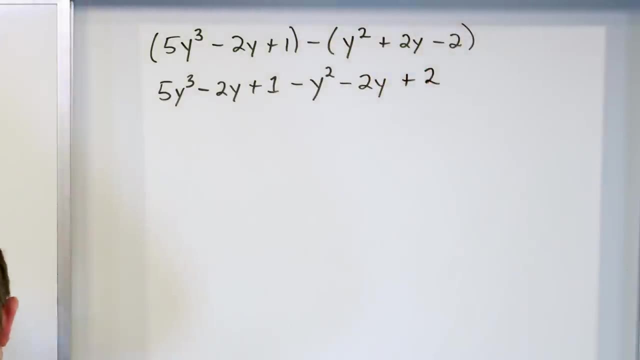 negative 1 times this, It's going to give you negative y squared. What is negative 1 times this, It'll be negative 2y. Negative 1 times negative 2 will give you positive 2.. So that's going to give you that, And then we'll switch over and say: look for like terms. 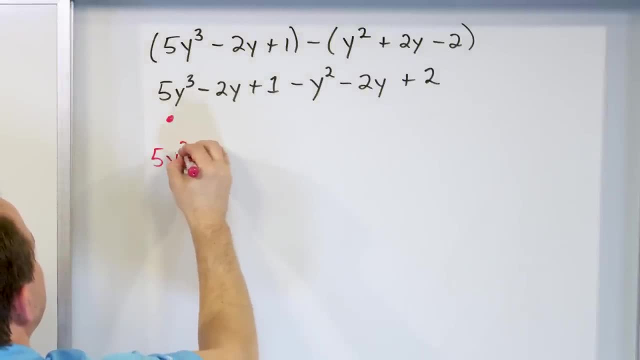 Here's a y cubed. We don't have any more of those, So we'll have y 5y cubed. We have y squared here. We don't have any other of those, So we'll have negative y squared Then. 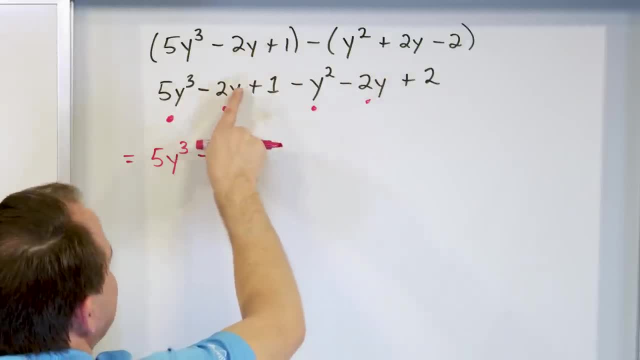 we look at y terms: Here's a y term, Here's a y term, But now it's negative 2 minus another 2.. So negative 2 plus a negative 2. So you get negative 4y, Negative 2 plus negative. 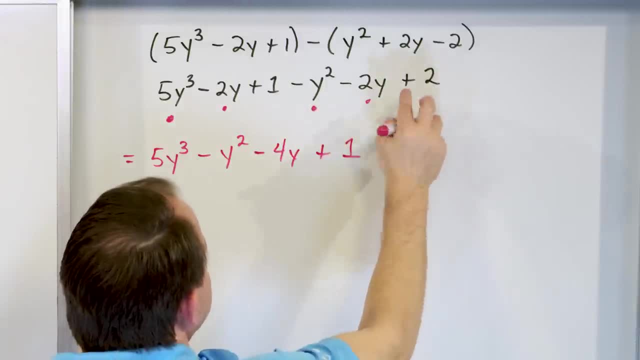 2 gives you negative 4. And then you have the plus 1 from negative 2 plus negative 2. And then you have the plus 1 from here and the plus 2 from here. So the final answer will be 5y cubed minus y squared. 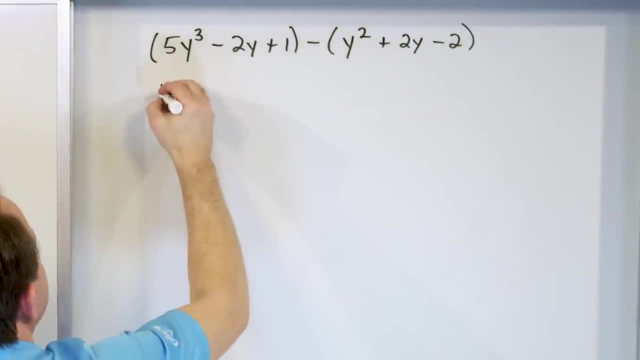 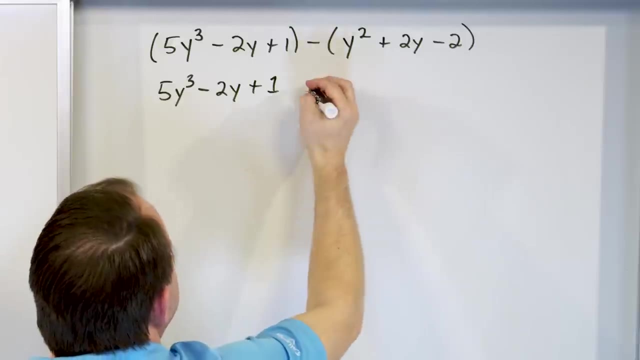 which means we have to distribute this negative one in. So let's go ahead and do that: Five y cubed minus two y plus one. What is negative one times this? It's going to give you negative y squared. What is negative one times this. 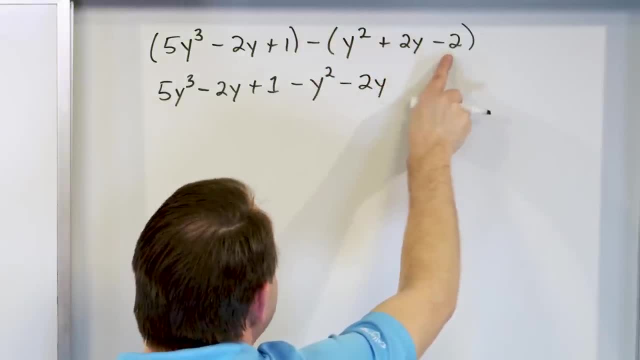 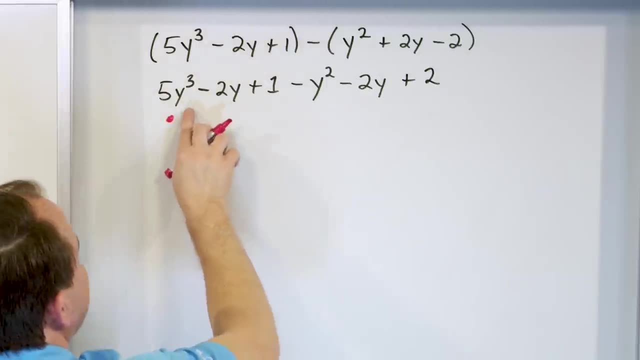 It's going to be negative two, y Negative one times negative two will give you positive two. So that's going to give you that. And then we'll switch over and say: look for like terms. Here's a y cubed. We don't have any more of those. 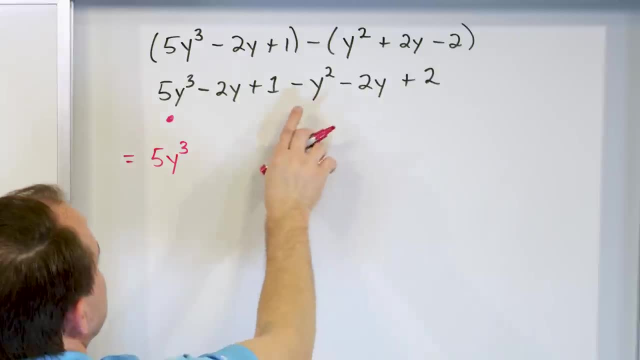 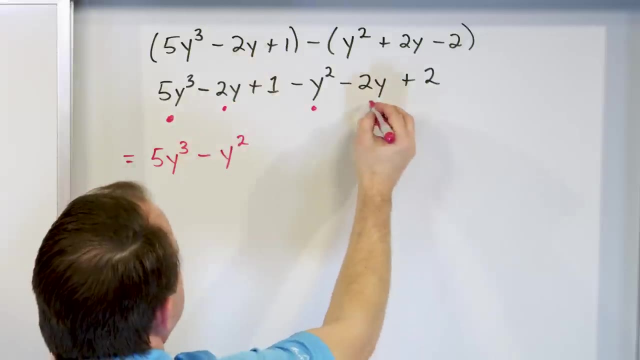 So we'll have five y cubed. We have y squared here, We don't have any other of those, So we'll have negative y squared. Then we look at y terms. Here's a y term. Here's a y term. 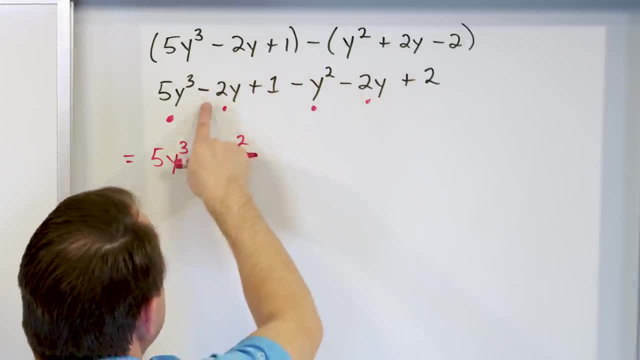 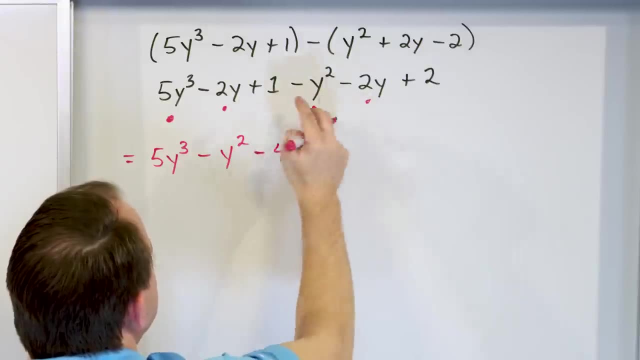 But now it's negative two minus another two. So negative two plus a negative two, So you get negative four, y Negative two plus a negative two gives you negative four, And then you have the plus one from here and the plus two from here. 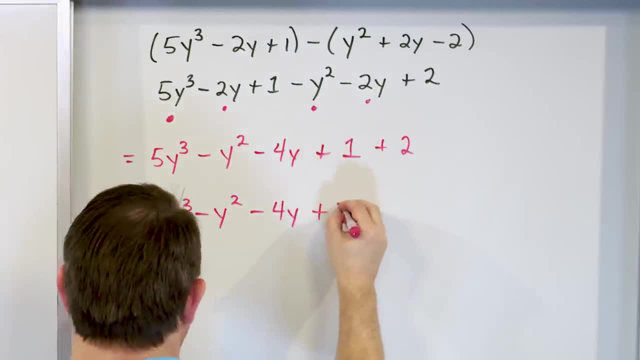 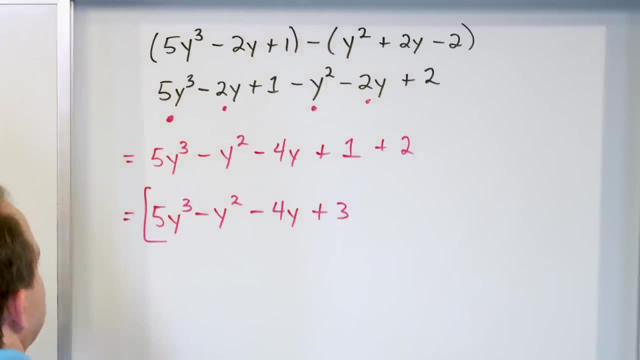 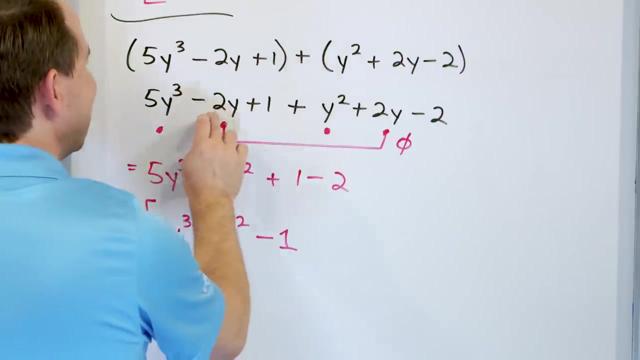 minus 4y and then plus 3.. 5y cubed minus y, squared minus 4y plus 3.. And notice that this is different than before. We only had three terms in the previous, because in the previous, because of the way it all worked out, we actually had a cancellation, which means we add to. 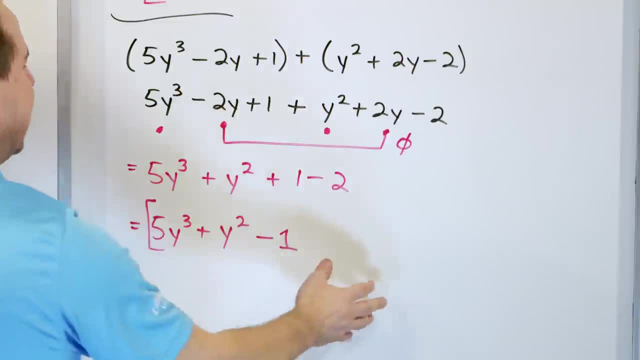 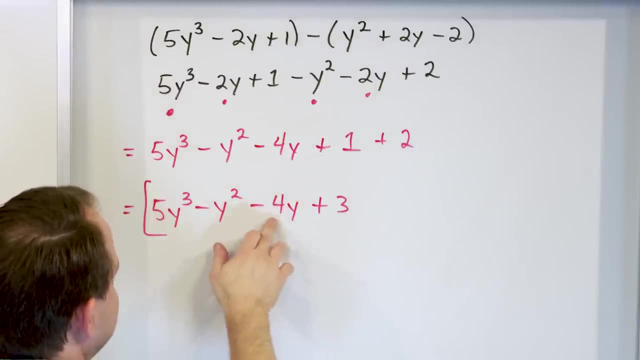 zero. So those y terms drop away. There are no terms, just in y. So we're going to have negative 4y. But when we change it to subtraction, they ended up adding together- or subtracting however you want to think about it, to give you negative 4y. 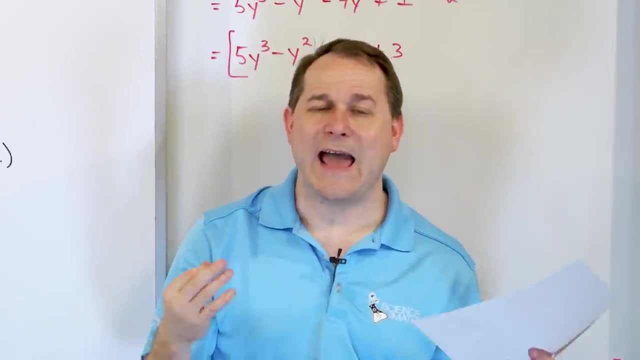 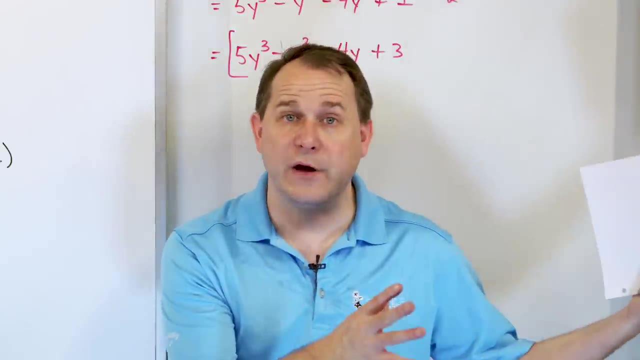 So it goes without saying polynomials are really important. And adding polynomials is really important because you're going to find out that lots and lots of problems in real science and math you might have one function over here that's a polynomial And you might.